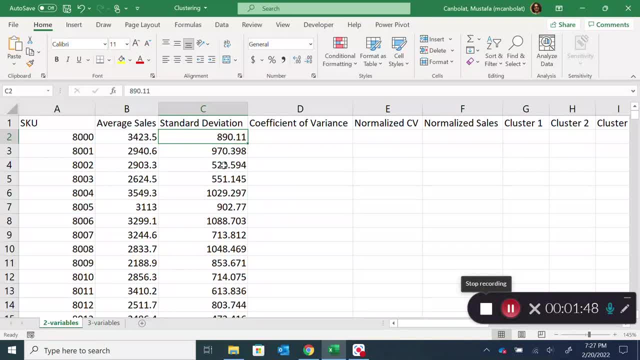 the average value. it makes sense. It kind of explains or just provides you the magnitude of the standard deviation compared to in relation to the sales amounts. You can think that as, for example, if you have 10,000 as the sales and the standard deviation 100, which is kind of small. 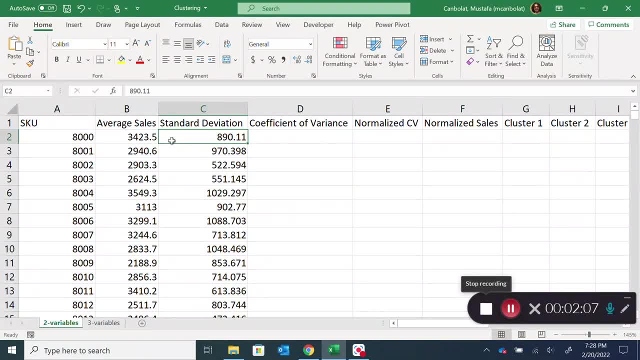 but if you have sales 100 and standard deviation 100, which is kind of large. So in that case, instead of using the standard deviation, you may want to use the coefficient of variance, which is the standard deviation divided by the average of sales, which is the ratio of the. 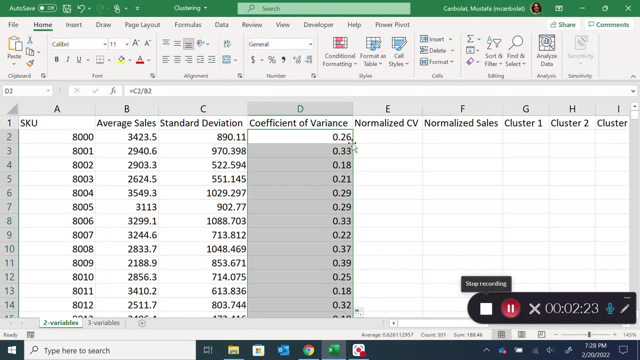 standard deviation by the sales. So this is now. these are the numbers that we have found for the coefficient of variance. So if I look at the average sales and the coefficient of variance now and using these two information, I want to classify my observations. So I may be able to do that by: 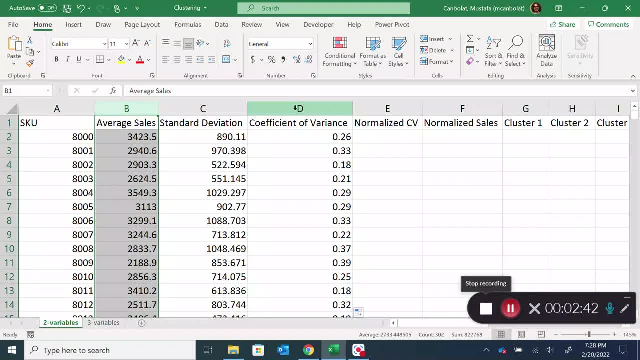 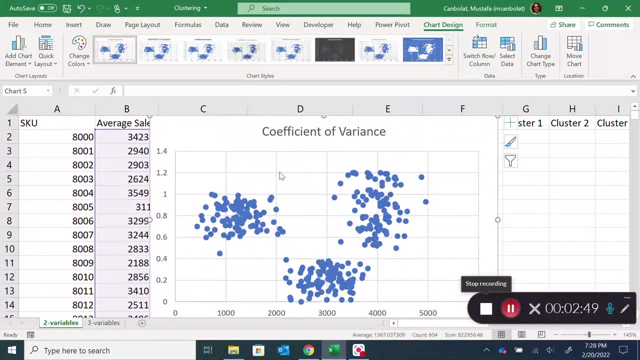 just creating a scatter chart And I can just create a scatter chart for these two columns And I'm able to see that there are three distinct groups. Why? Because I created this data set myself. It is a synthetic data set, It is not a real data set. 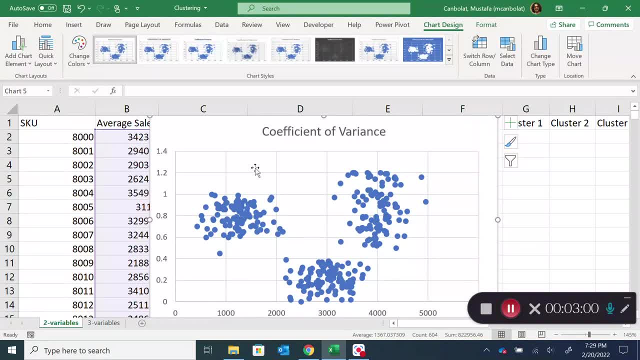 And now I have to explore the idea. It looks like there are eyes and the nose possibly. So what's happening here is that I want to find the cluster means And because there are only two variables, I can see that. I can see that there are three distinct clusters here. 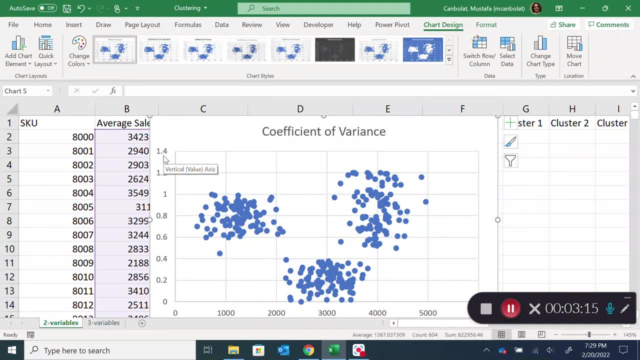 But what if there are more than two variables? If there are three variables, you are not going to be able to see. this cluster means Then maybe you need a 3D plot. What if there are more than three variables? So you're not going to be able to see that. 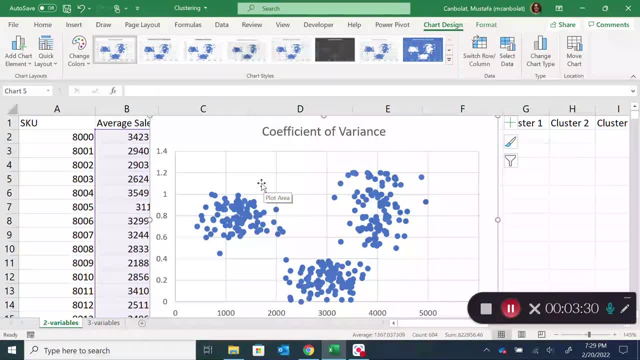 to visualize that and that is going to be difficult for you to kind of identify the number of clusters or the cluster centers, etc. You need an algorithm to do that. So in that case, for the algorithm to work, what we need is we need to standardize. 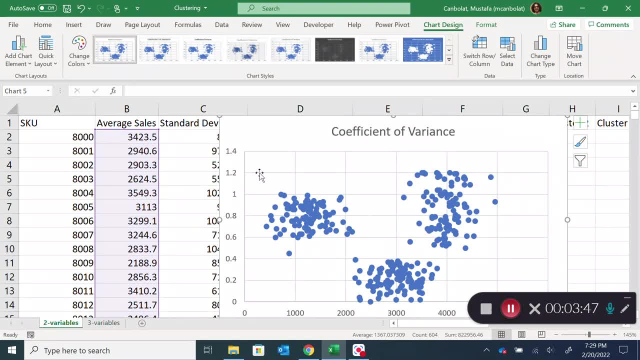 this variable. So here the coefficient of variance happens between 0 and 1.2,. but these observations, the sales amounts are in thousands. So if I look at the distance between, for example, these two points here on the x-axis, maybe 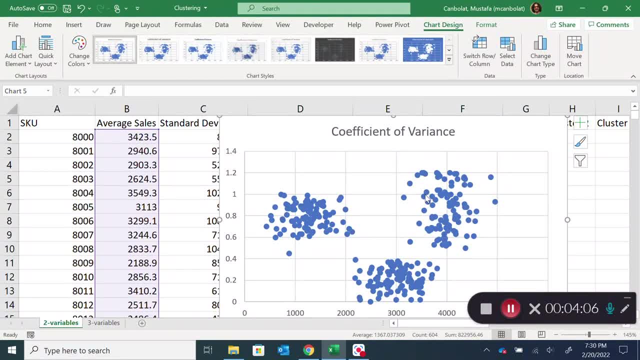 it's about 100 or something like that, But on the y-axis this is less than 1, maybe 0.1 or even less than 0.1.. So if I want to try to find the distance from any center of a cluster, here to the points, 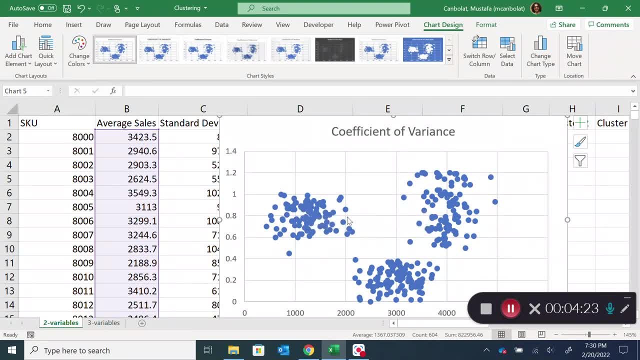 and I am going to favor the x-distance over the y-distance. and I will not really care about the y-distances at all because they are very minimal, So I will only pay attention. the algorithm is going to put all the emphasis on the x-distances, not the y-distances. 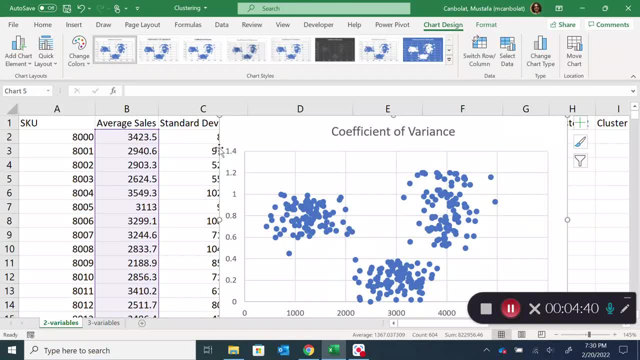 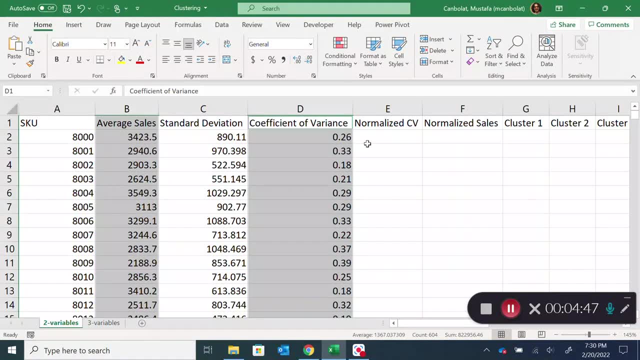 and that is going to create wrong results. So what we need to do is we need to standardize these variable observation values first, before running the algorithm. So how do we do that in Excel? We just use the function standardize and then it is. 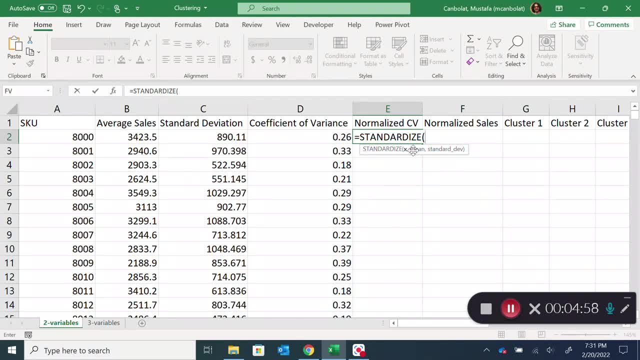 going to use the x, which is the values and then the mean of that column of that variable and the standard deviation of that variable. So let me just name that first. okay, So here are my sales. So I just use ctrl, shift and down arrow. 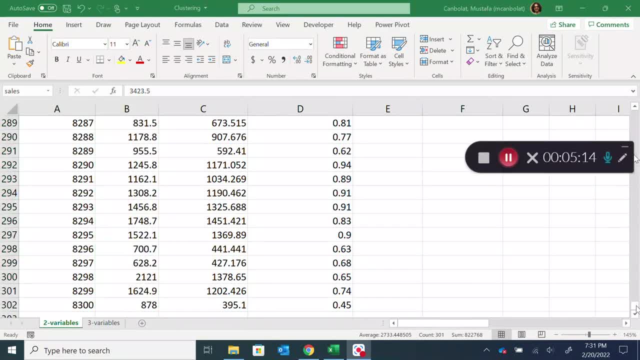 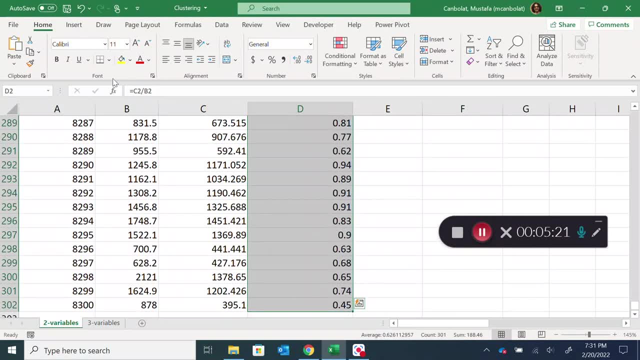 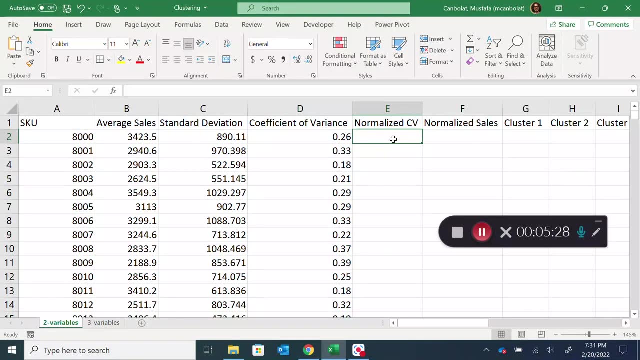 then these are named as sales. Okay, it's already there. And then I'm going to also name the coefficient of variance. I may also have that. It's not there, Okay, so that is going to be cv. I'm going to name that, So in that case I can just 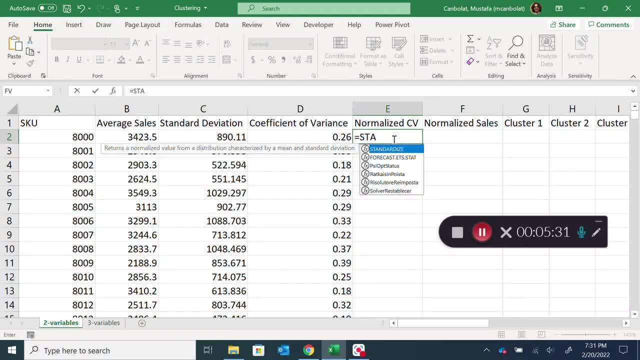 normalize my cv, the coefficient of variance: standardize, And the x is this value, The mean is the average of the cv and standard deviation of cv. Okay, Then I am done with that. I'm going to use the same idea for: 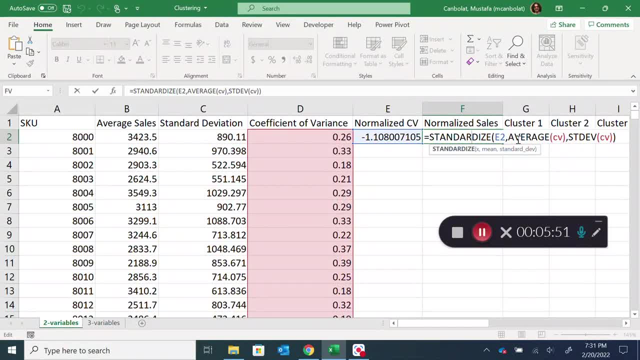 the normalized sales, And instead of using that column, I'm going to use average of sales And standard deviation of sales, And then this is going to be finding the average sales and then standard deviation of sales, but not this one. I'm going to be using what? 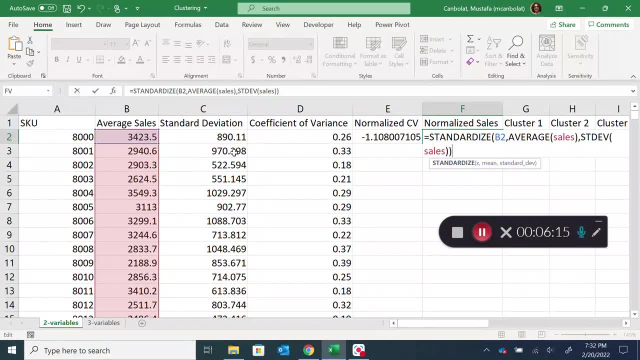 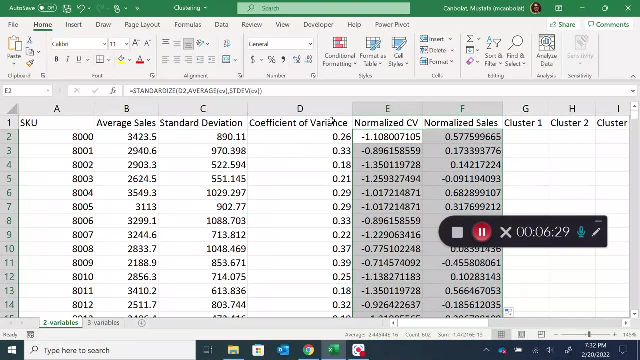 This value average sales here And sales, and then average sales and standard deviation of sales, So I am able to find my normalized sales values as well. Then I'm going to double click on that and find my normalized coefficient of variance and sales values. 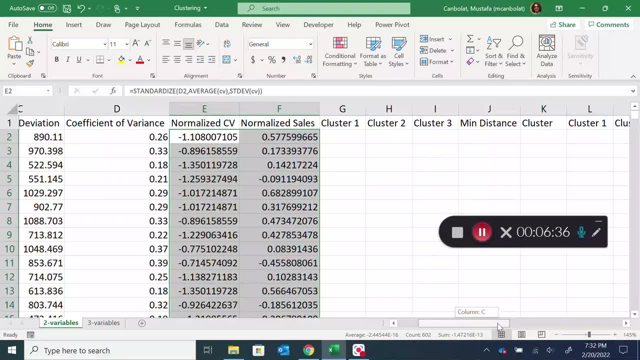 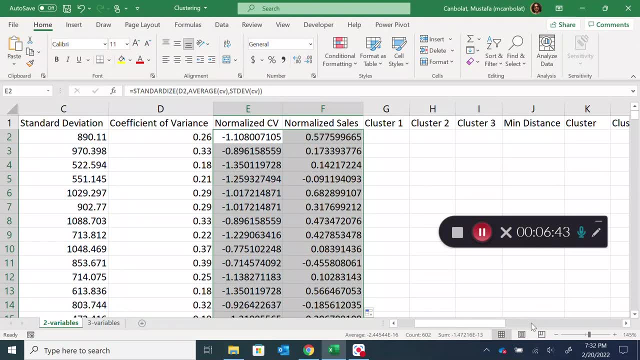 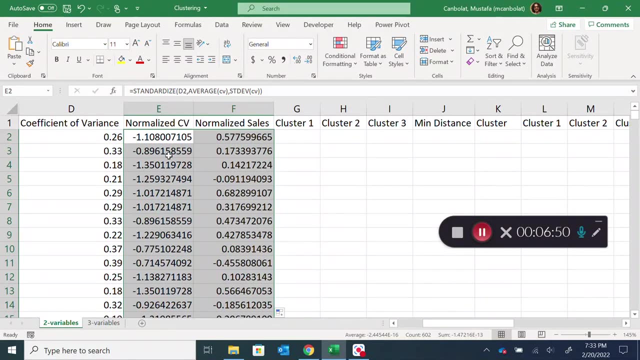 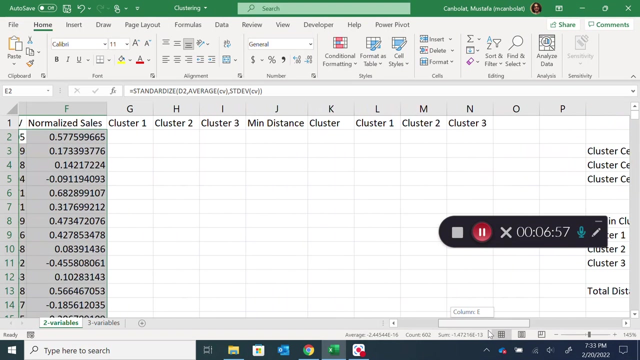 Now I can just go ahead and identify my clusters using these values, not the original values, So distances are not going to be very far away from each other in terms of their scale here, So we could use this as standardized values. Now the problem with Excel is: I need to determine 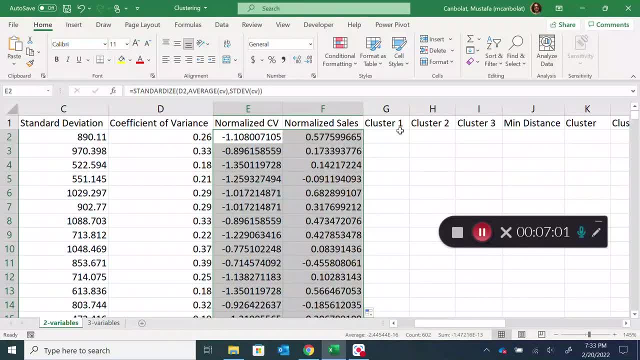 first start with the number of clusters. I decided that I want to use three clusters and I knew that the three clusters would be better to use, And this is the k-means clustering. So I decided that it's going to be a three-means clustering. 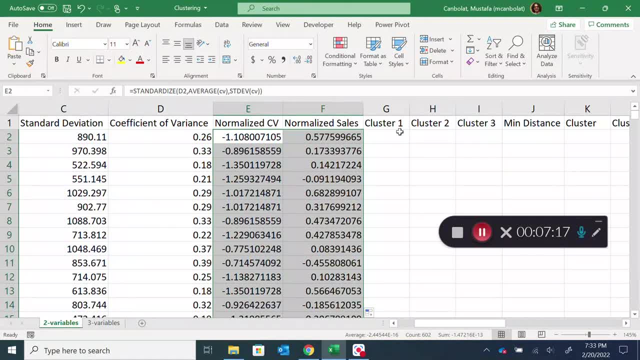 If you want to use Excel, then you'll have to do two clusters, three clusters, four clusters yourself, And if you use some other, maybe programs- you can do that in an easier way And you can also use hierarchical clustering as well. 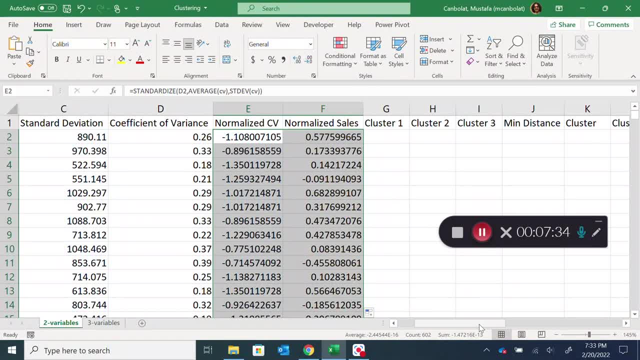 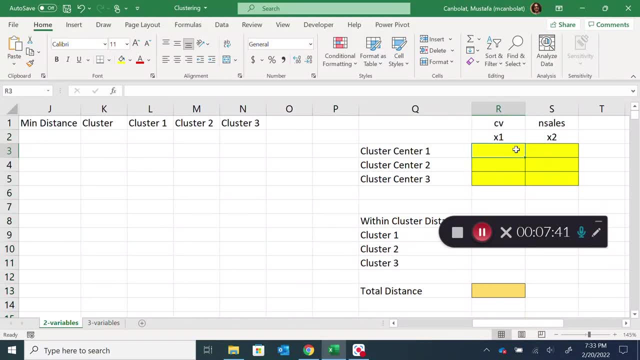 And you may be able to find the best number of clusters. But let's just try to understand that. we know that there are going to be three clusters And I want to put this cluster means, as one of them, 00. So these are kind of initial starting points for the cluster centers. 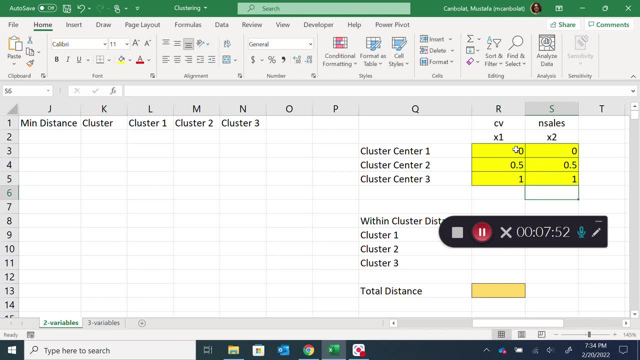 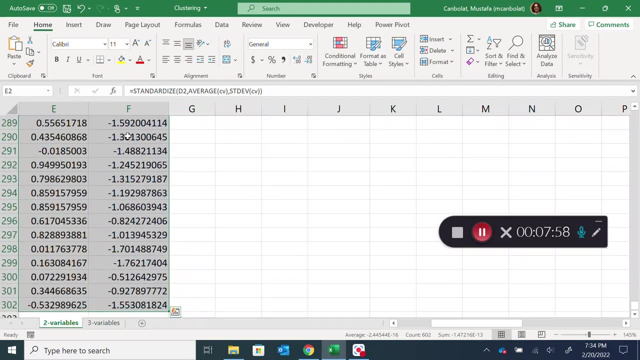 And what I want to do is I want to find the distance of each observation that I have. I'm going to use this to let me just color them with your favorite color. Which one is favorite color of yours right now? Let's just do green. 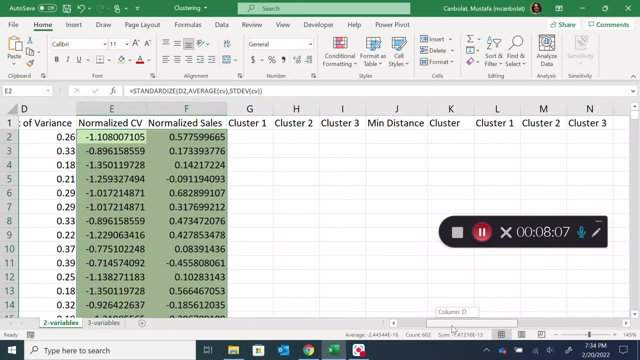 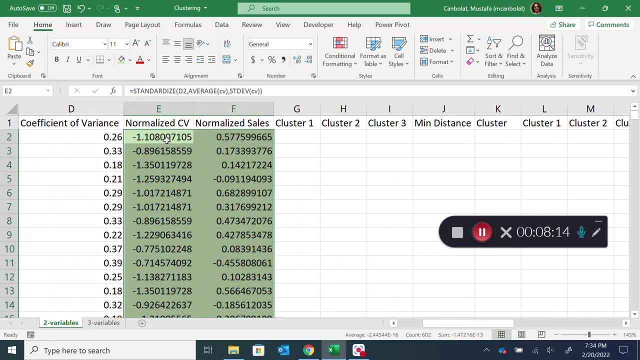 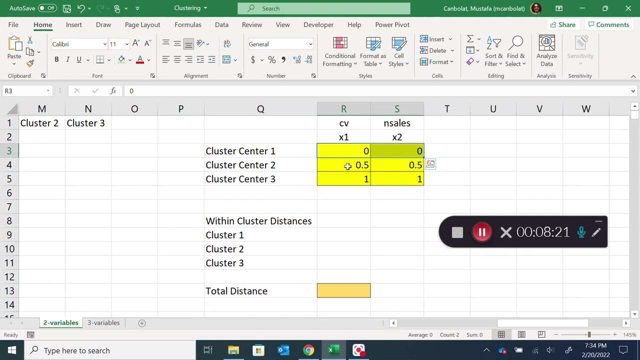 Okay, So what I'm going to do is I'm going to use this tool and I'll find the direct distance, So Euclidean distance, from this observation to this center and then calculate for the second center, the third center, and then i'm going to just decide which cluster, center or which cluster to use. 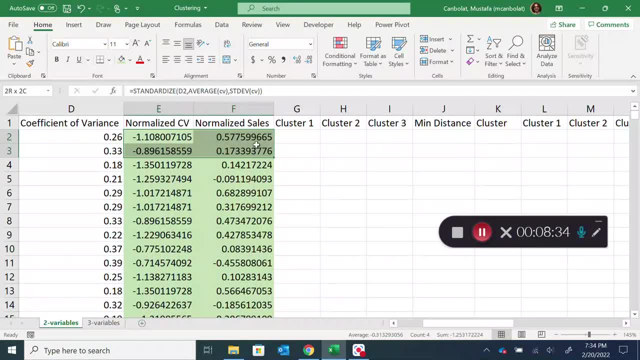 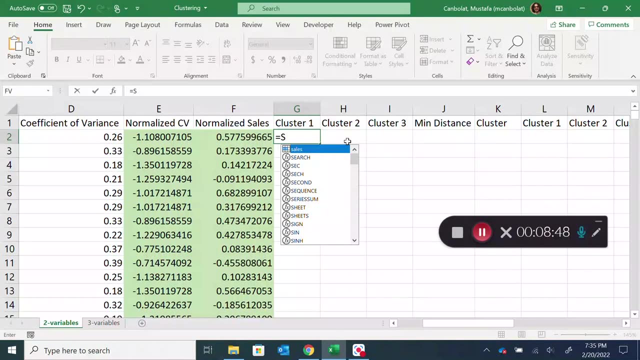 for that, uh, for that observation. so i'm going to assign a cluster to this point based on the minimum distance. so i do that is, i'm going to use the, the euclidean distance, the direct distance is square root of what i'm doing here. sqrt of this cv value, the normalized cva value minus the cvs. 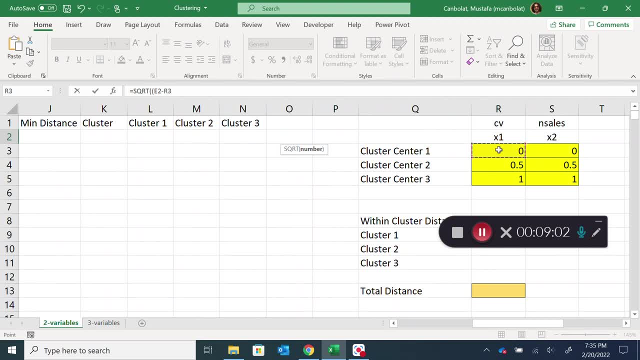 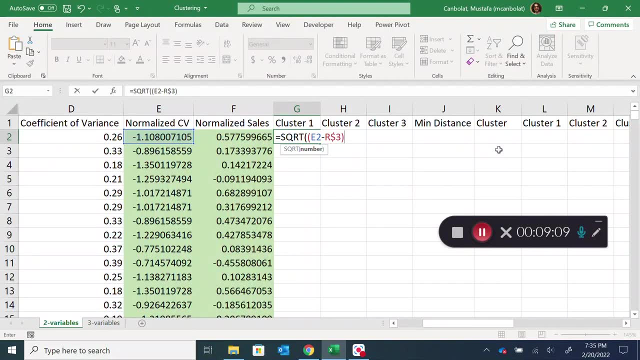 center for the first cluster, and then i'm going to put a dollar sign on that. okay, and only that one. and then i'm going to square that. this is i'm finding the euclidean distance plus. i'll find this one minus the second center and put my dollar sign on it so that when i copy and 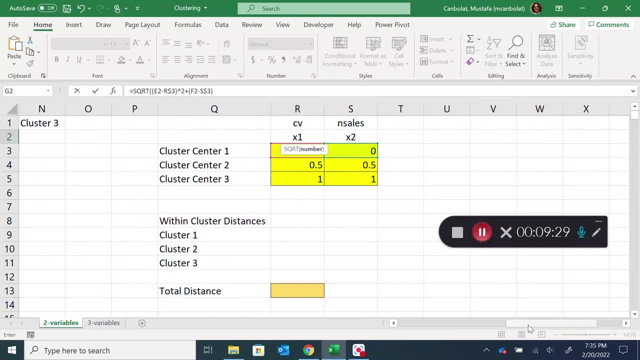 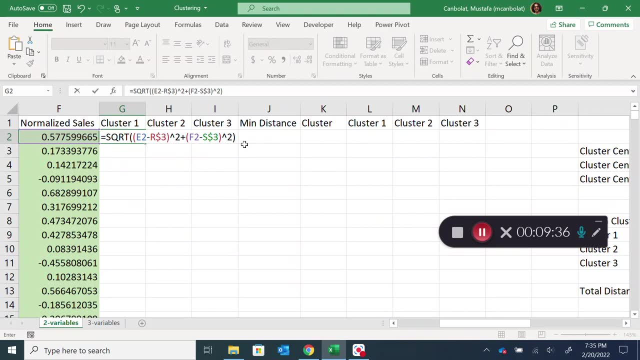 paste. this does not go down, okay, and then, once that's done, i'm going to square that and that's. both of them are going to be under the square root. if there are more than two variables, you can continue adding these and finding three dimensional distance or four dimensional distance. 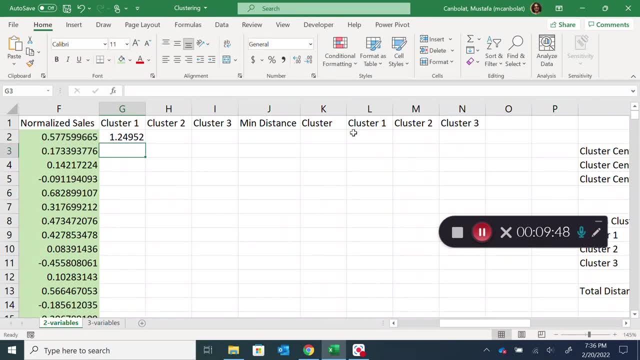 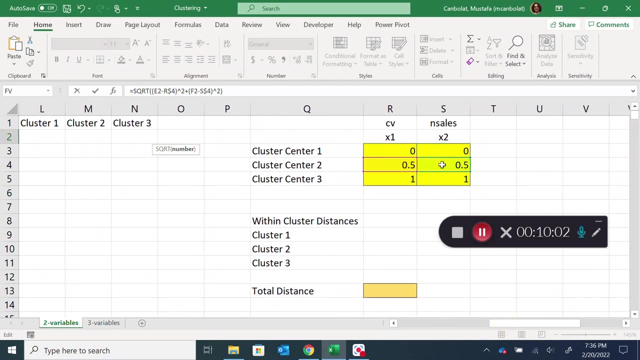 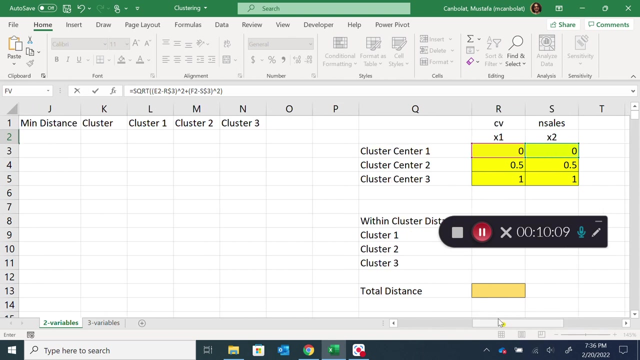 etc. so it's just enlarging your square root function there. okay, so this is the cluster, and let me just copy this here and i'm going to just change this to now i'm going to use this: two cluster center values and then for cluster three, and it is going to be this, the third one. okay, and that's done. 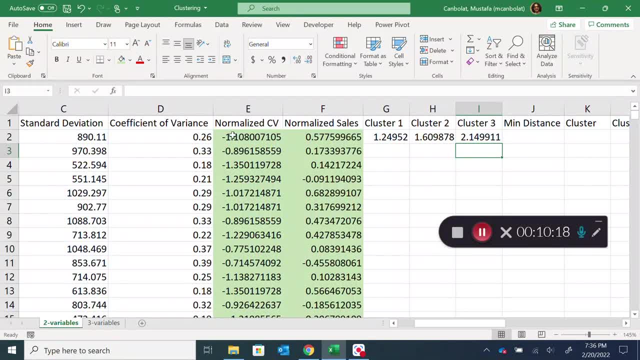 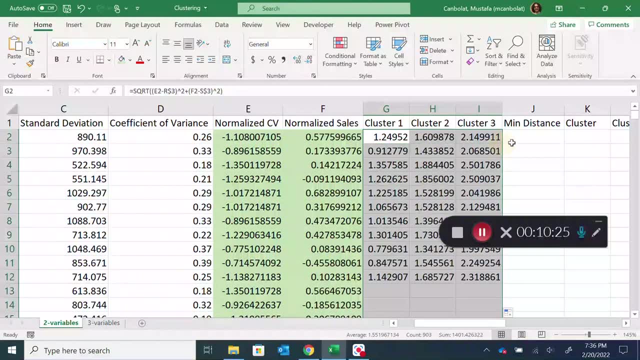 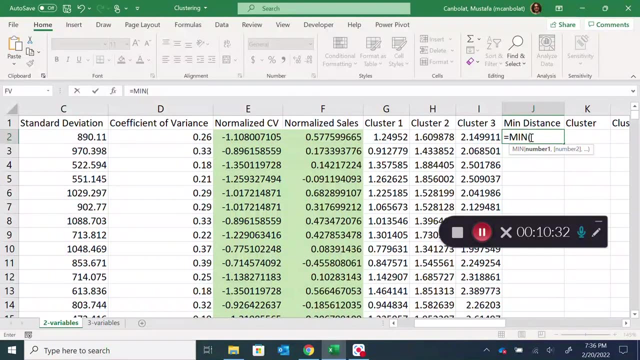 and i'm able to find the distance from the this point to the first cluster, in the second cluster and the third cluster, and for every observation i found them, then i'm going to use the minimum of this three and the minimum is going to be 1.249. 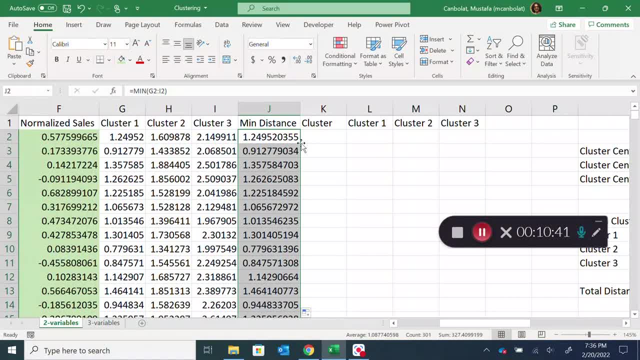 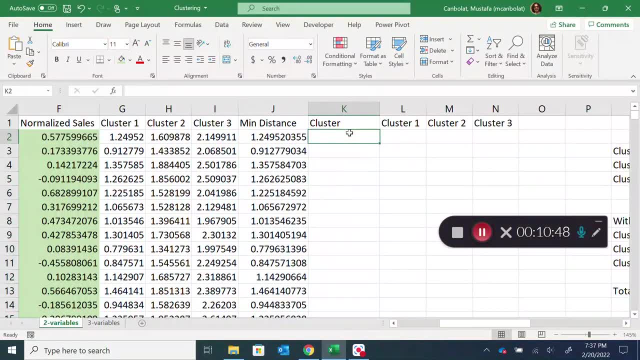 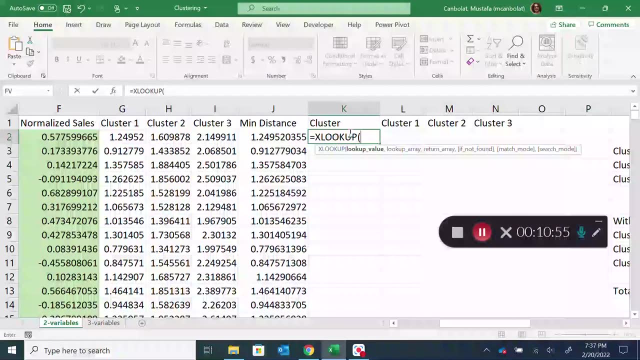 and i'm able to find the minimum distance, and we are able to find the minimum distances for every one of them. so it's time to assign the cluster so you can use two different functions. one of them is xlookup, which is a new function and maybe some excel versions would not have it. it's easier. 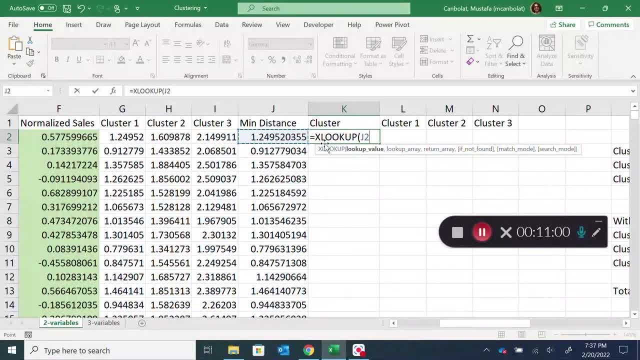 to use. i'll just say 1.24 here. that's a lookup value i'm looking for in this range here and once i find them, i'm going to return the value of the matching value from here. and then the next thing is: if not found, there is nothing, i'm not going to do anything because we're going to be able to find. 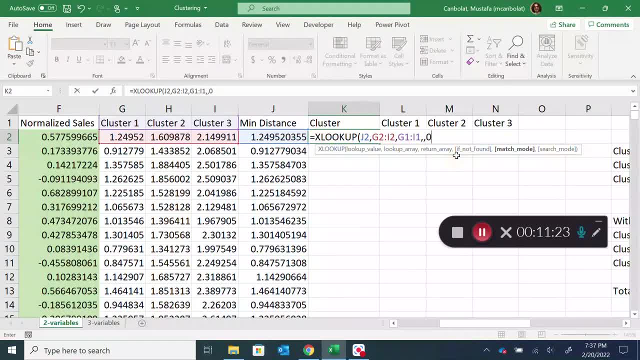 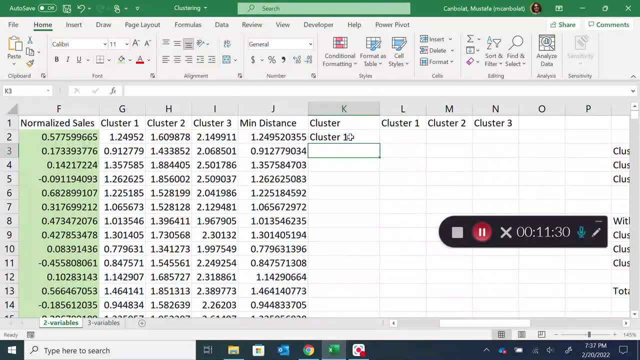 it and match is going to be an exact match. and then the search model. i'm going to assume that's going to be default and done so, the cluster one. and for g2 and i2 and g1 and i1, i'm going to use my dollar signs here so that when i copy and paste this selection will not move down. 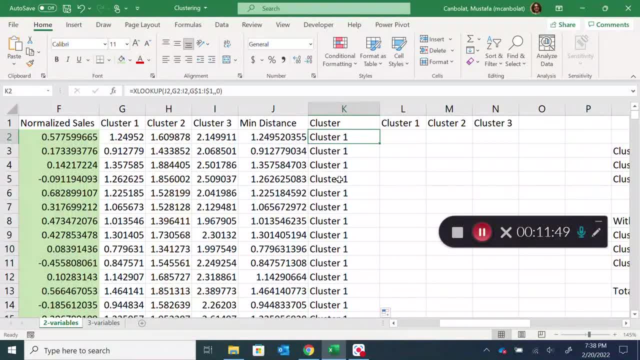 so when i do that, what happened here? so was it? this is also selected, and then it was able to find that it is still the shortest distance to cluster one. and is it all assigned to cluster one? no, so the formula works and, but it is not the correct assignment. 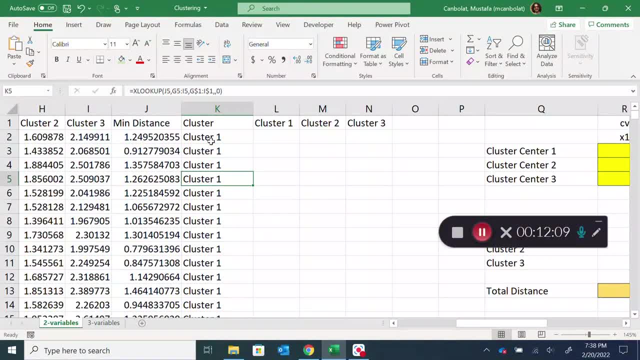 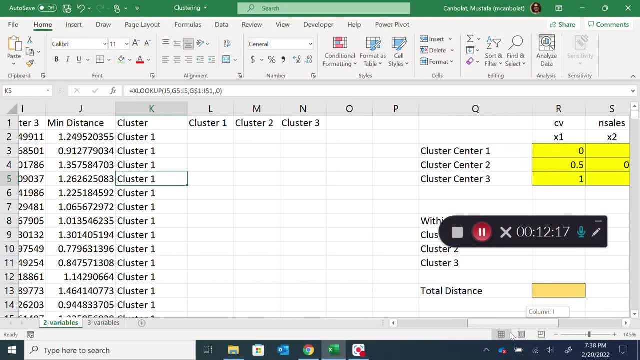 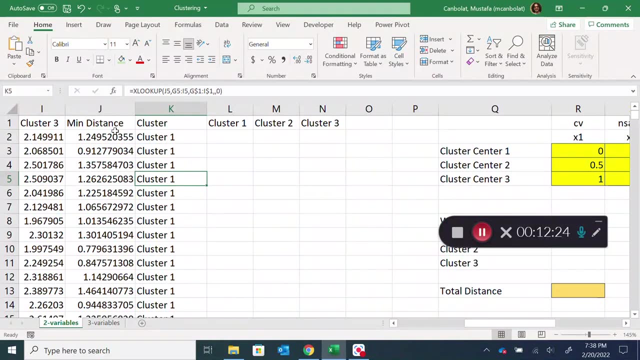 okay, that means now we were able to put the clusters in there based on the minimum distances. now if we change this cluster centers, then the assignments of these clusters are going to change and be based on the minimum distance. think that like maybe, uh, you are putting the retail. 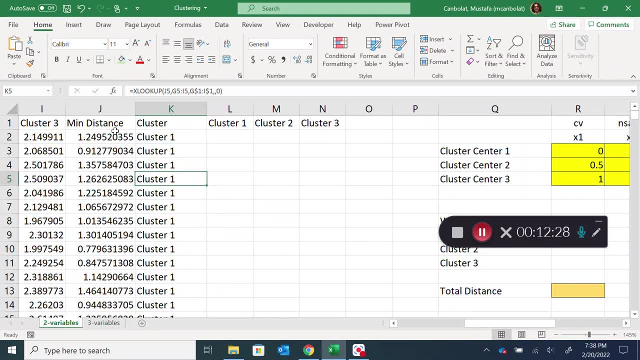 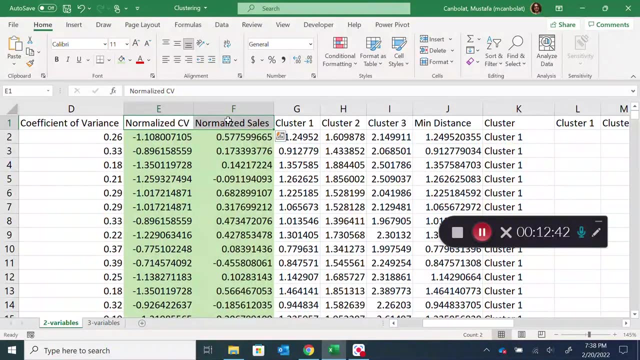 centers and you're trying to find a distribution center to assign for those and find a location for a distribution center and you can do the same thing. okay, now i want to just visualize this, and how do i visualize is that i want to look at this normalized cv and normalized sales values. 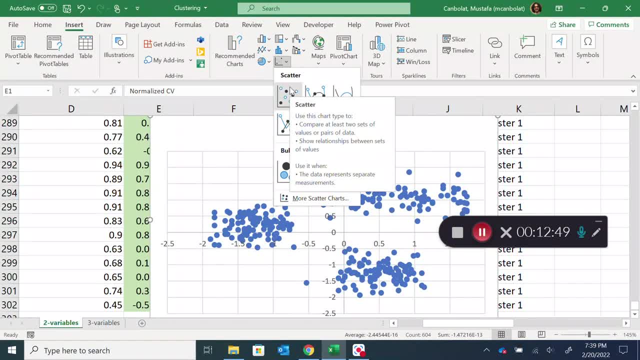 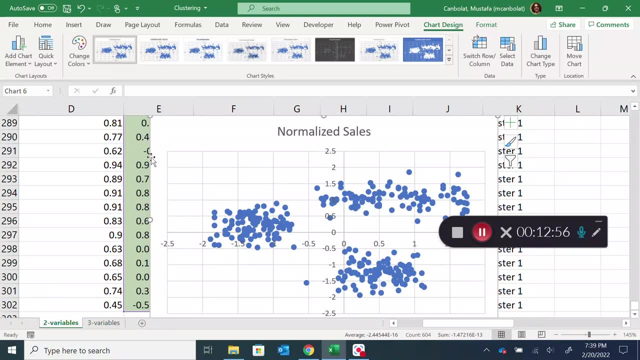 and i want to create a scattered chart, but i what i want to do is i want to display them in different colors just to illustrate that the assignment of these clusters- i know that the perfect assignment is going to be three distinct colors for this, three distinct groups. 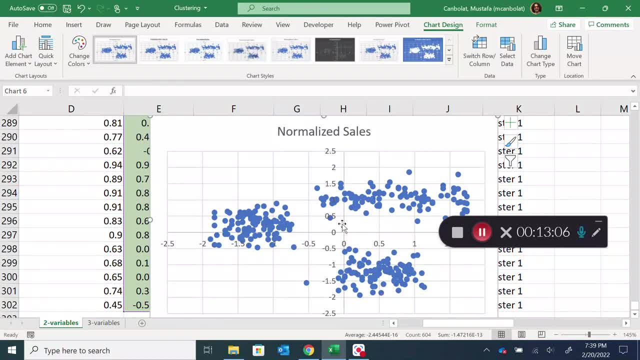 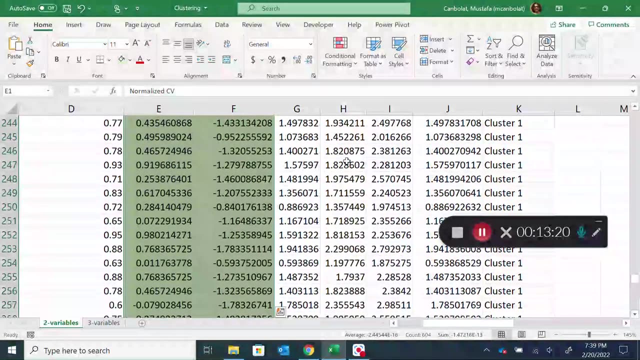 but that may not be the case because we have wrong. cluster means one of them is zero, zero, one is 0.5.5 and the other one is 1: 1 and none of them are closer to these points here. so that means what we have to do is we have to use and just to color them. it's not going to work, if you also 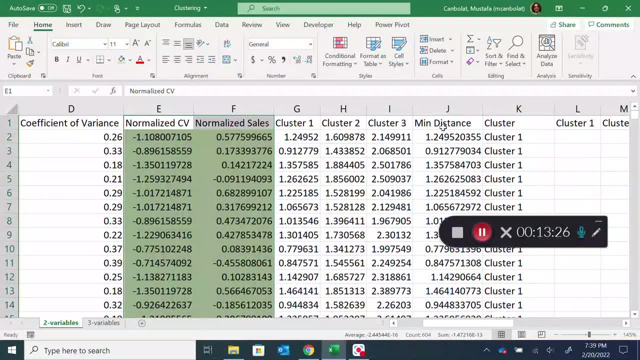 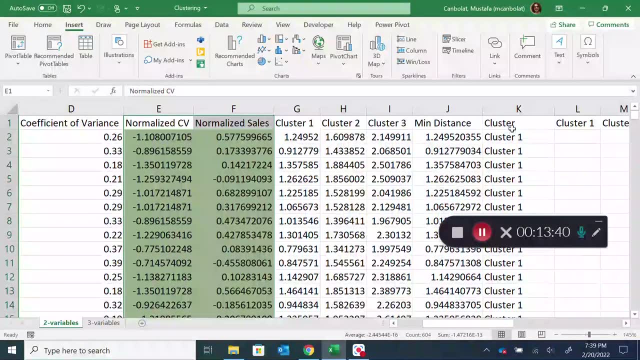 highlight these clusters and then put your uh scatter diagram, which is the. the shame for microsoft. they haven't really put the um, the scatter charts with the distinct colors, using the legends, and we have to do uh, maybe, uh, an approach that is going to be a fix for that. 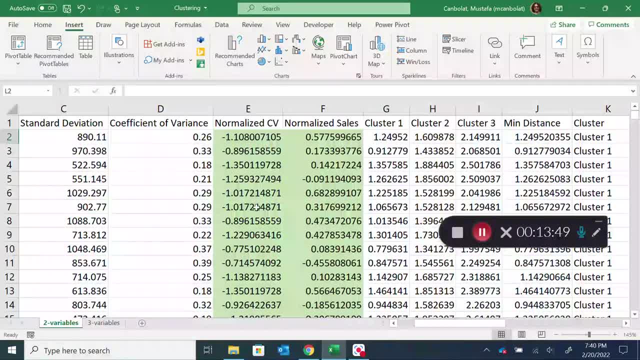 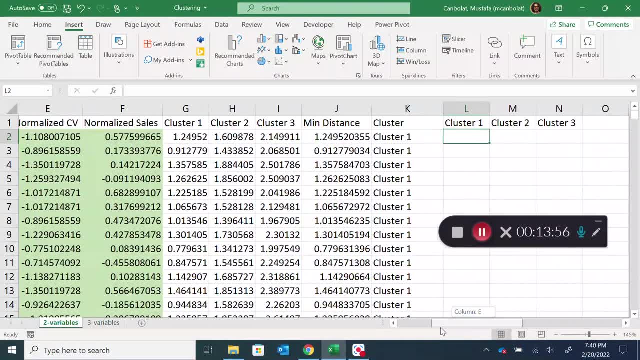 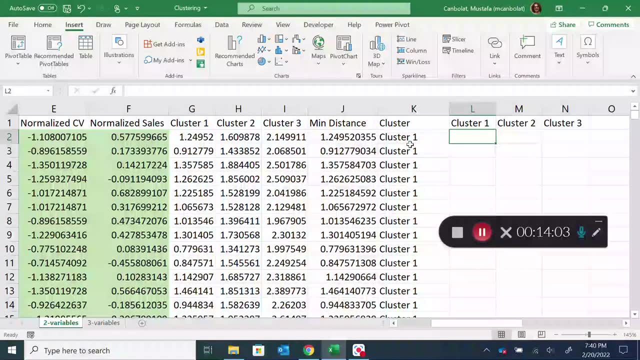 so what we need to do is we are trying to find the cv versus the sales for each cluster. that means what we're going to do is we are going to display the the normalized sales only for that specific cluster. so we need to put the sales amount for cluster one here and maybe if it shows cluster two we will put. 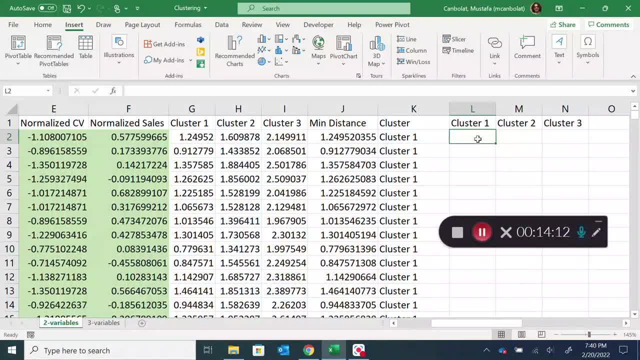 the sales amount in here. so to do that i'm going to use the if function, if okay. so if this cluster is equal to here, then the result is going to be the normalized sales. otherwise the result is going to be na. so we need to put an na function here, otherwise if you just put a blank, 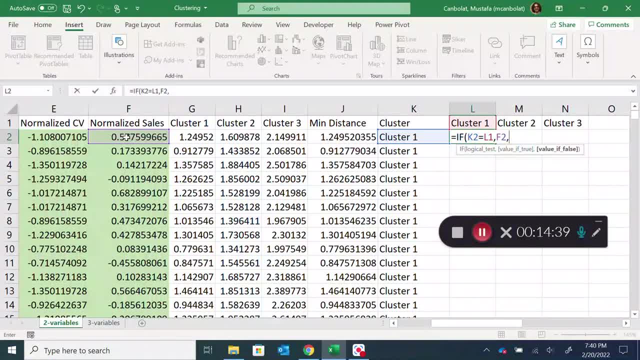 it is not going to work. okay, that means we'll have to just put the na function, which is another shame for microsoft- just fix this. and what we have to do now is we need to put our dollar signs in the correct order, and if you don't know how to use the dollar signs, i have another. 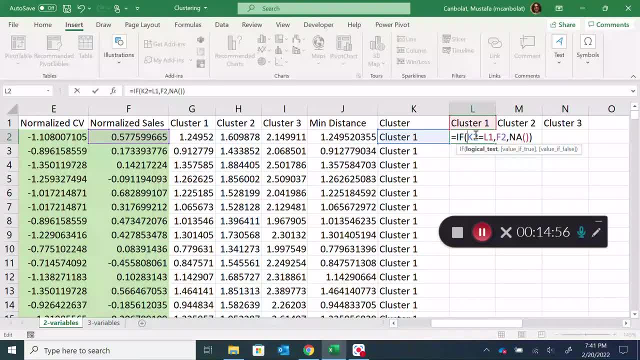 video that you could first, uh, look at that video and learn about the dollar sign usage and then come back here after. so i'm going to put the k2- this one should go down, but not to the right. so it is going to be dollar, k2, l, m and when i copy across this one should just to be copied across, but it should. 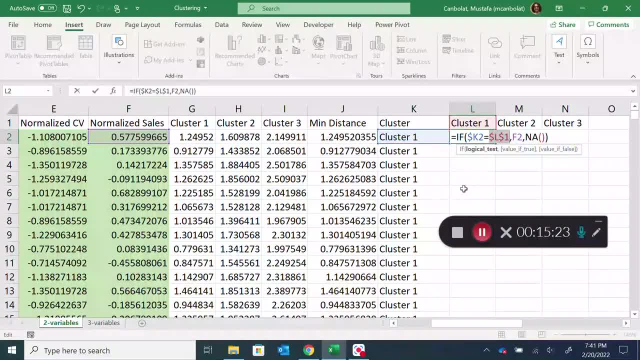 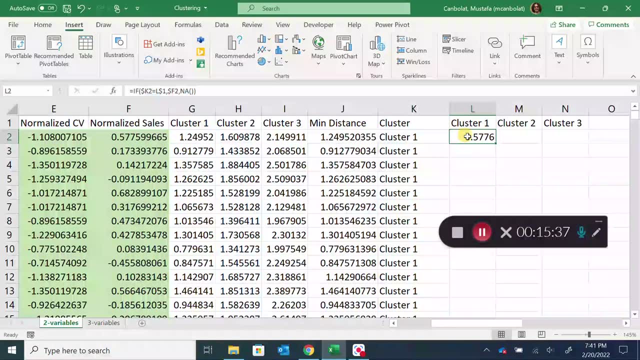 not go down when i copy down. so this is going to be l dollar one and f2. we want this to go down but not across, so that is going to be again the holder f2 and it's done. so. this because it shows cluster one. here it shows the value, but for cluster two and three it shows n a. 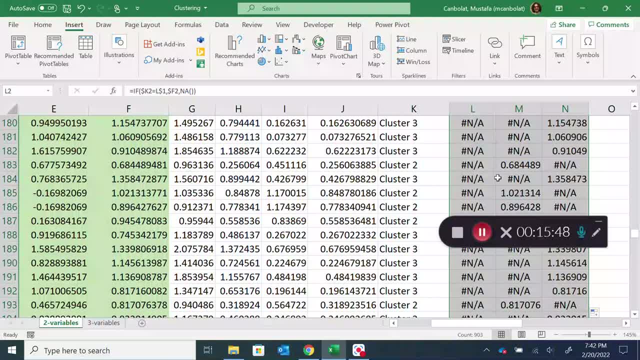 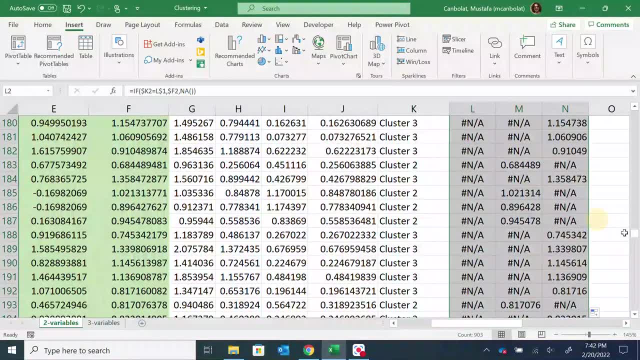 and now we're able to do that. if you look at down here, this is cluster three and the value of the m sales and normalized sales is displayed for cluster three. okay, and if you are logged in, you do not runにos b2 instead of nostats in configuration, so you 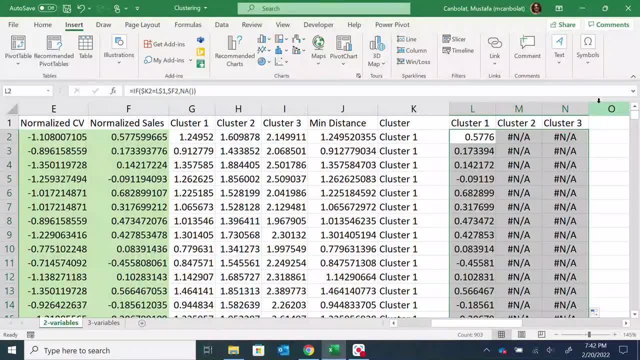 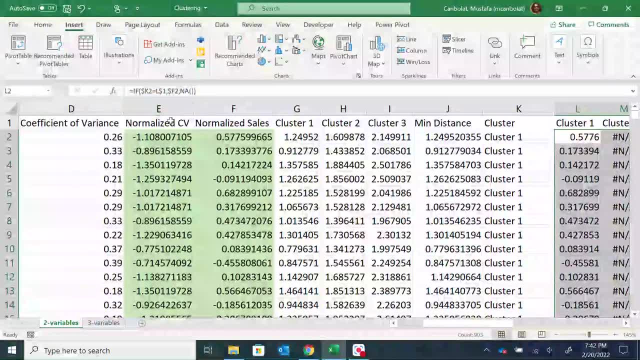 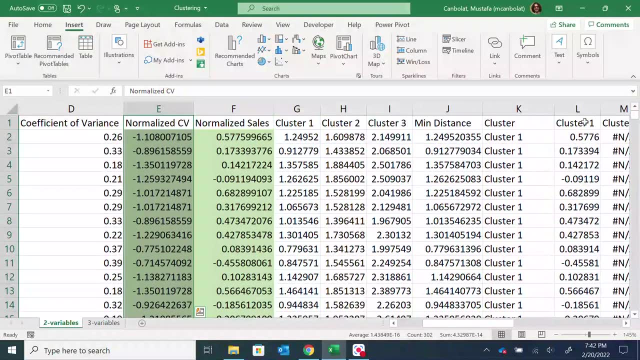 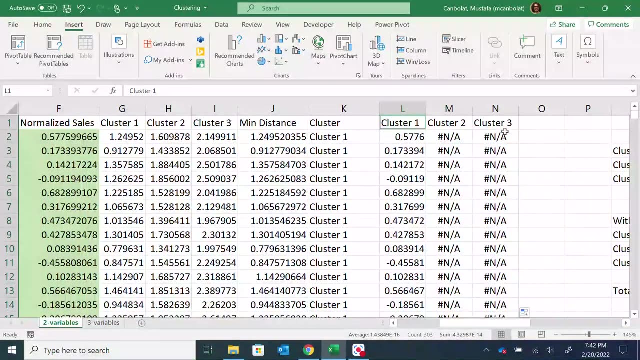 And if you have difficult understanding this, you can pause the video and maybe try to understand it before proceeding. And this is just to display my clusters here. So I'm going to highlight the normalized CV values And then I'm going to press control and highlight this three here. 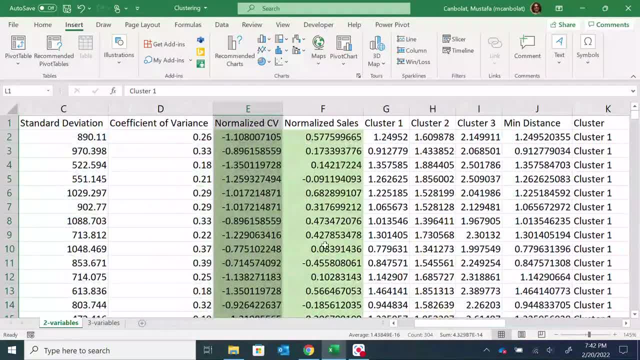 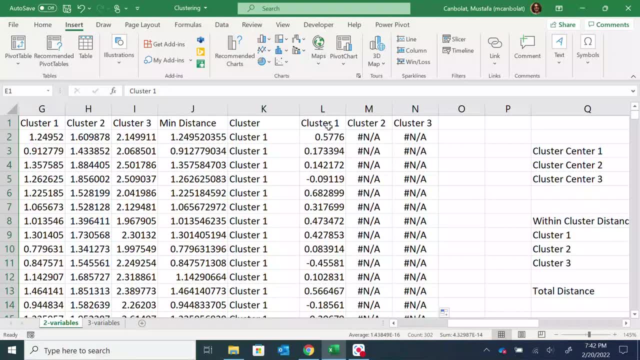 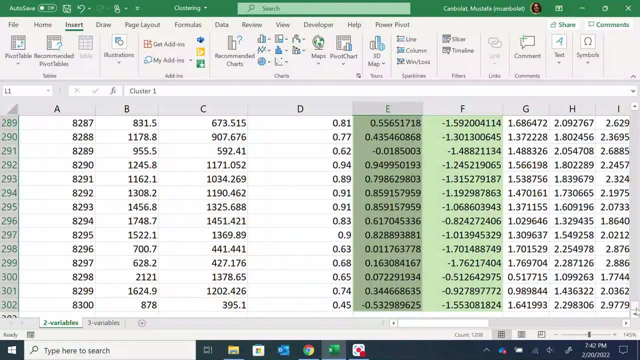 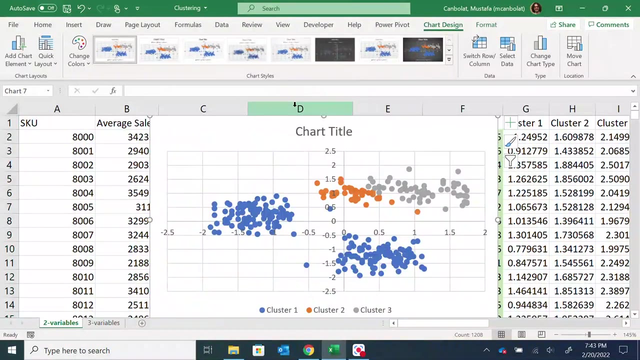 Okay, let's just do this one more time. Normalized CV values are highlighted And then the clusters are highlighted as well. Then I'm going to control shift and down arrow. So I have highlighted three columns there and one column here, And look at the beauty now, this kind of chart. 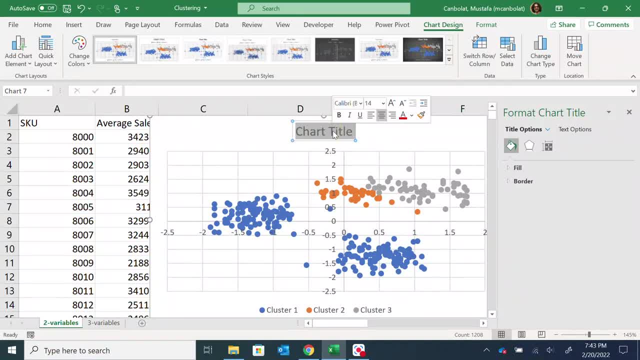 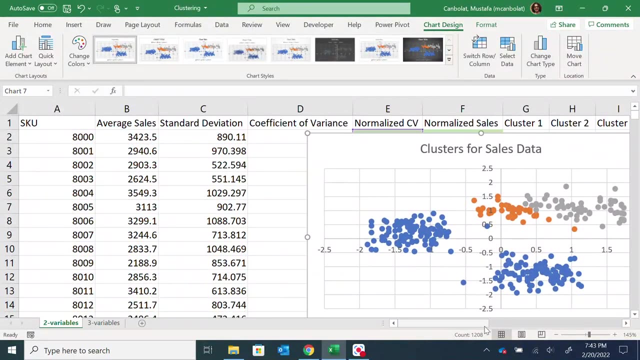 So we were able to find the clusters For sales data, Okay, good, And this is not a correct set of clusters, because what's happening here is we have the wrong data to start with. I mean the wrong values to start with, not the data. 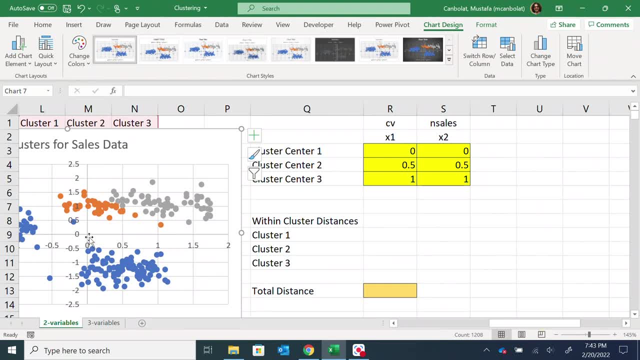 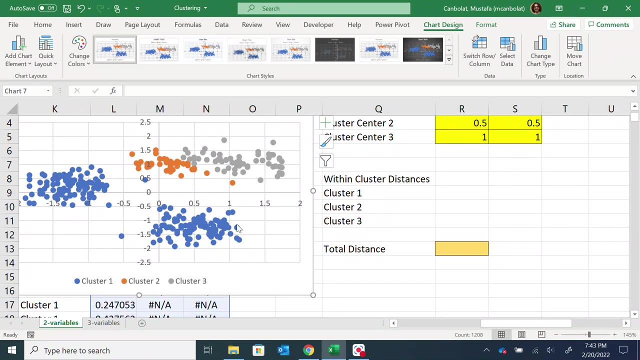 So here, what's happening here is that for 0,, 0, this point here, And it is assigning all the points, The blue points, right? So that's the cluster center one And it's assigned all these points to this center. 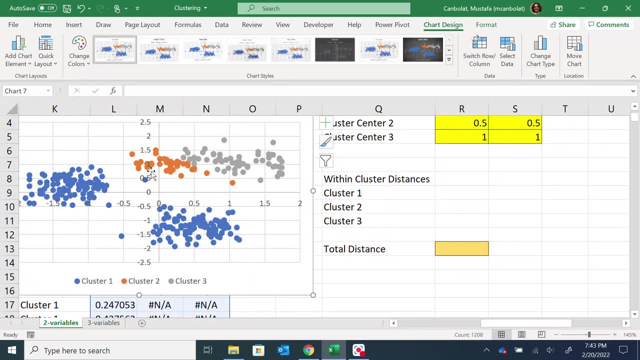 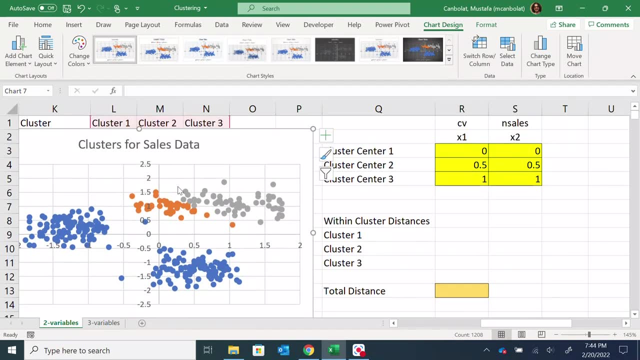 And then it assigns these, the orange ones, into 0.5, 0.5. The center, And then one one center gets all these gray points. If I also want to put the centers there, it's going to take a little time. 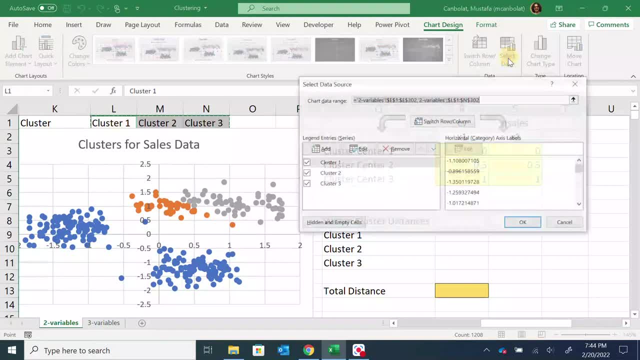 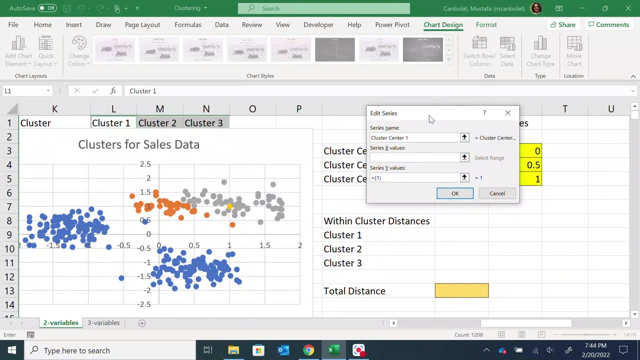 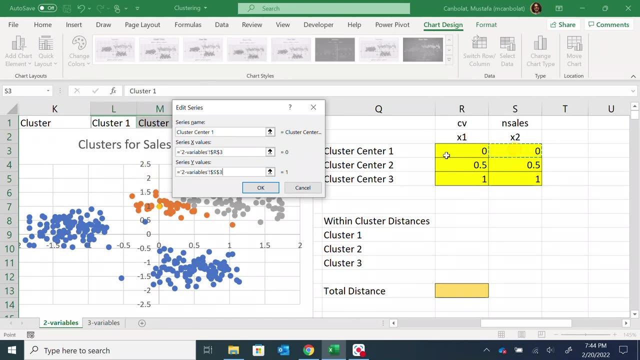 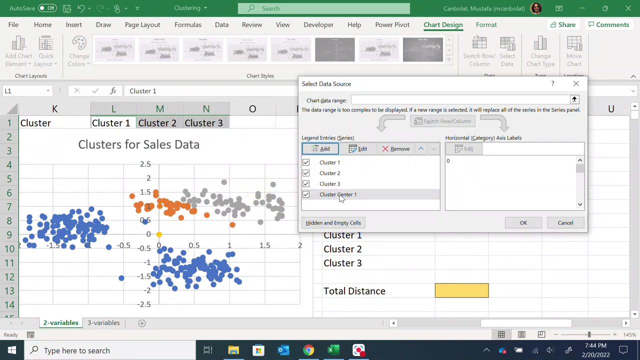 But let's just do that In various quick. i can just go to select data and add cluster center one and then the x values is going to be here, x, and the y value is going to be this, and i'm going to click ok, and i am able to find a cluster center zero, zero. that is for cluster center one. okay, 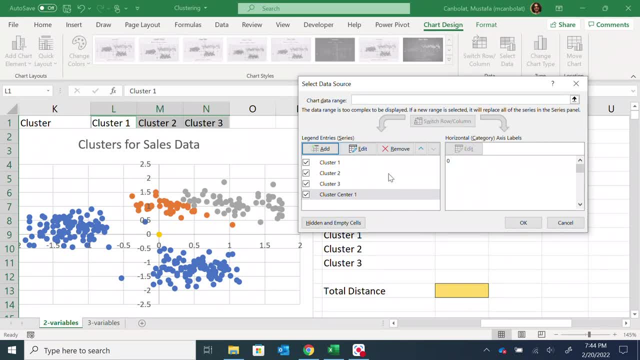 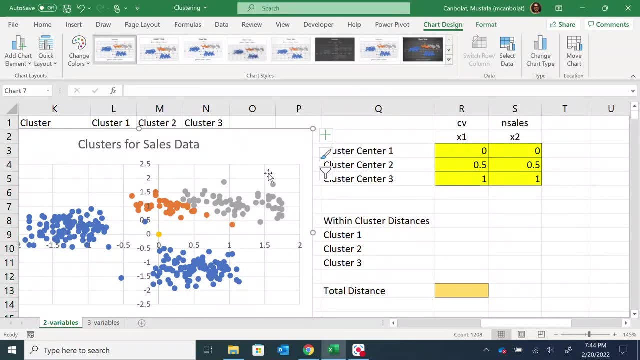 so i can do the same thing for cluster center two, cluster center three, and i'm gonna do that after pausing my video. let's first just maybe make an edit to that, and then i'll pause the video and then just add the other two. so for this one, just this one. i want to format this by just looking at: 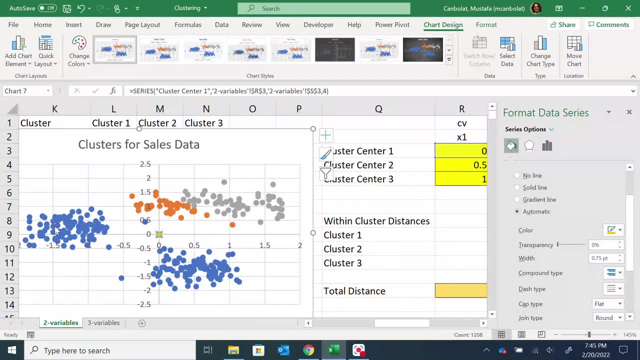 the marker and i'm going to make the marker the same color- blue. okay, so it's going to be blue colored marker and it is not going to be the same color as the marker. and i'm going to make the marker the same color as the marker and i'm going to make the marker the same color as the marker. 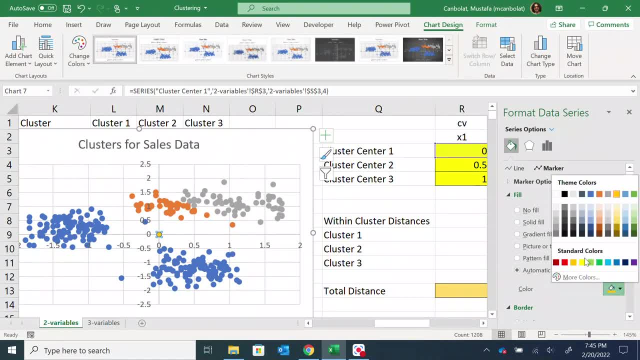 and it is not going to have a fill there- no fill. and what else i need to do here is that i want to make that larger and the marker options: i want to make a built-in marker with maybe one of this okay size- let's just make it 20.. 20 is a little big there, maybe 10. 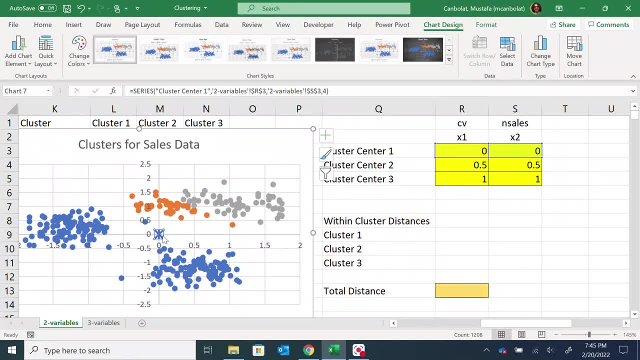 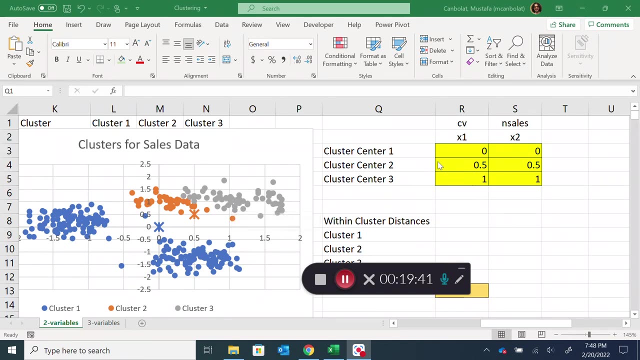 okay, good, so this is the cluster center for these points and i can just do the cluster center for the other two. i'm going to pause the video, do that and come back. okay, so i was able to just put those here. the gray one is hiding there, so maybe it's getting uh scared. so let me just try. 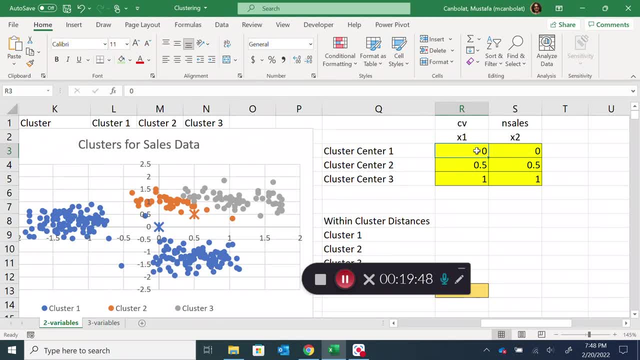 another uh. you know the cluster centers, so i'm going to use maybe negative uh one and then negative uh 0.8, something like that. what it does is now it put the cluster center there, assign now this point to this cluster. so the assignments have been changed and we can dynamically. 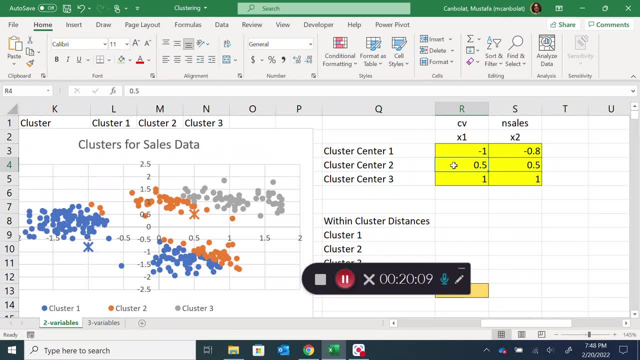 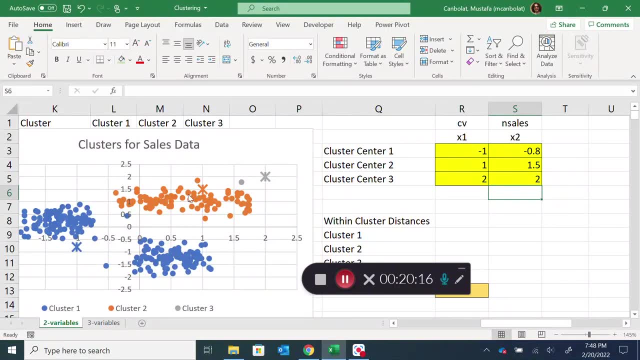 see those. let's say this is going to be uh one and one, point five and maybe two and two. so we are seeing now that it is not the best way of clustering, but it is just illustrating the idea. so in that case, what we want to do now is we want to be able to find this total distances from each uh cluster. 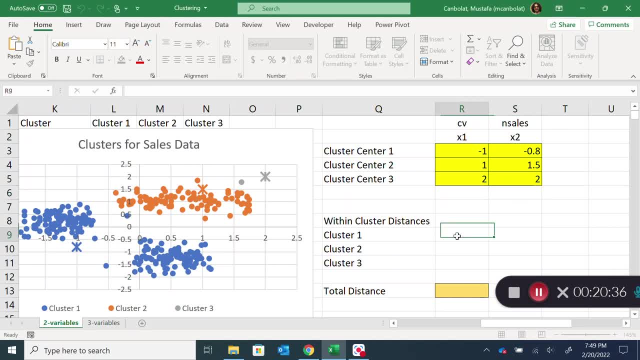 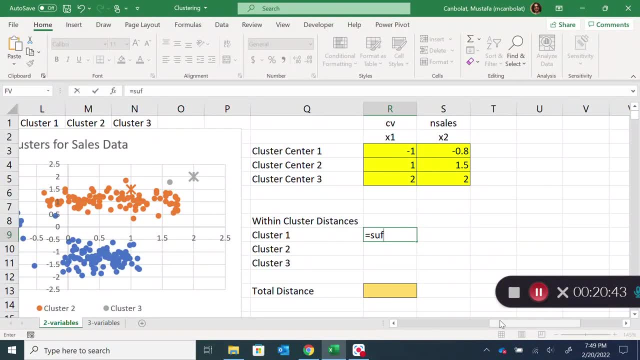 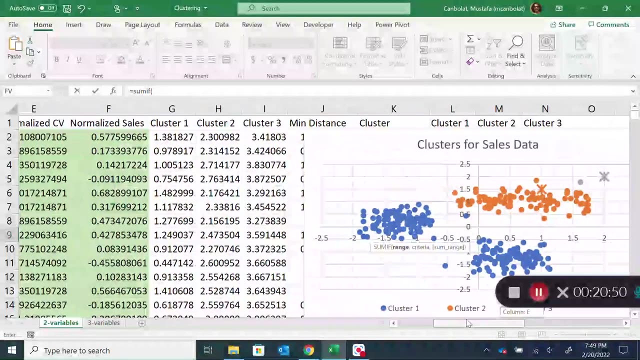 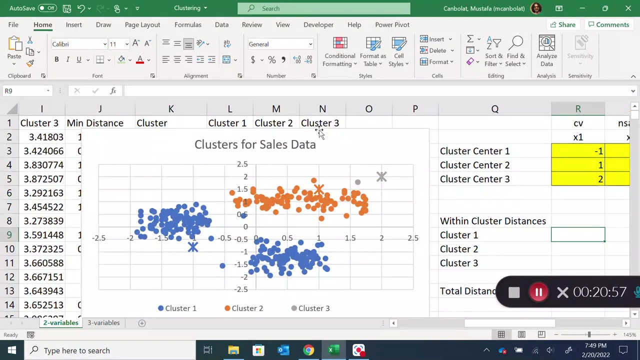 okay, and the assignments from the cluster to the points that are assigned to that cluster. and we'll find that by just using this sum if, function and some if is going to take this range criteria and some range. so the range is the, the clusters. so move this a little farther away here so that this graph is not really going to affect us. 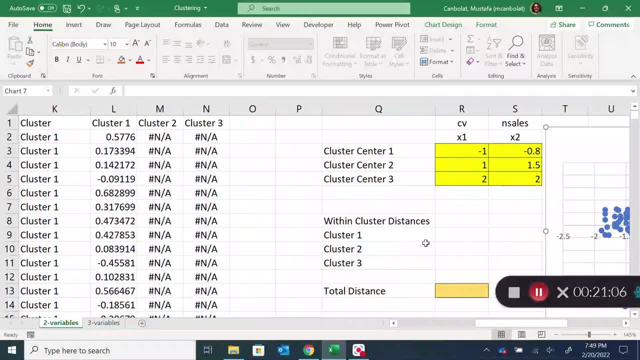 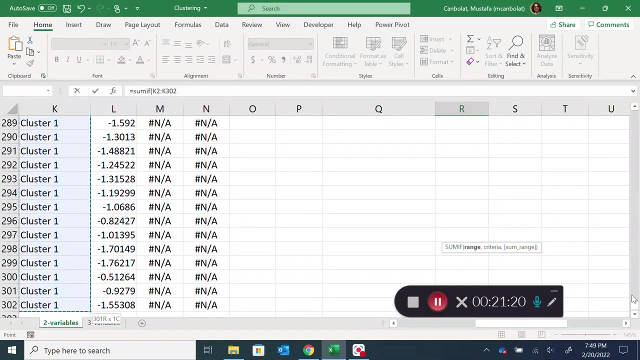 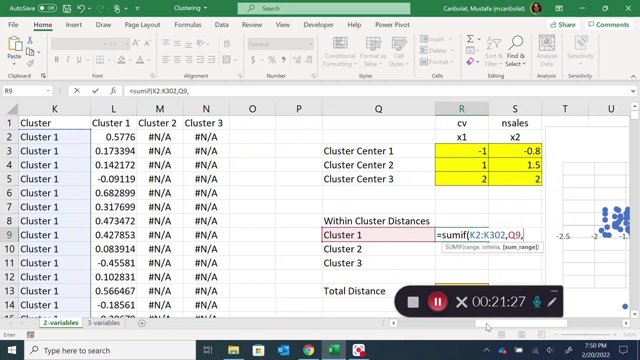 okay, so let's put that there. and now we could just do this. we are going to use sum if the range is these plus all these clusters there. okay, and then that's that right. here is cluster one, and the sum range is going to be the minimum distances. 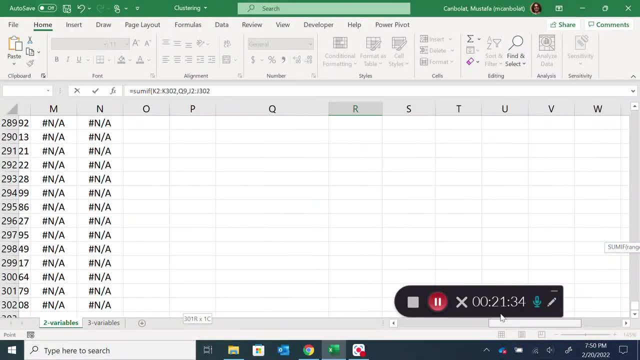 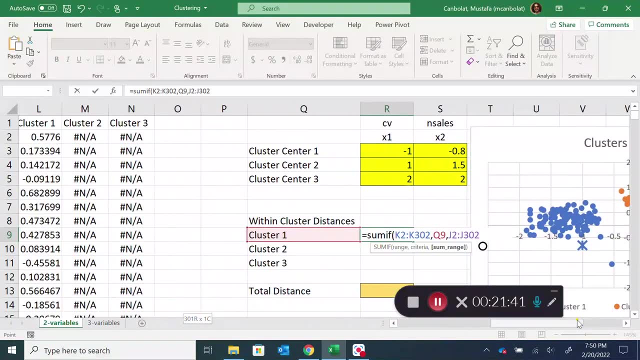 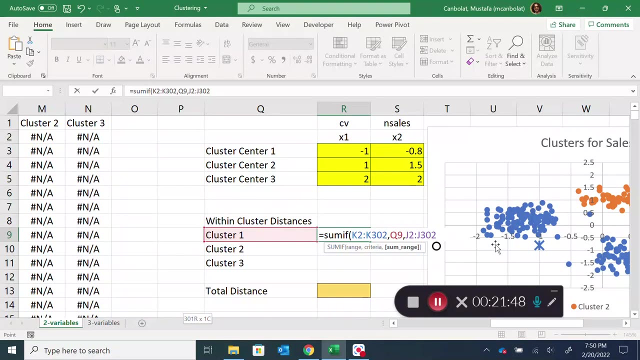 okay, that is going to give us the distances for only the points from this cluster center to every point there. okay, so that is now. i want to put my dollar signs on this- the dollar signs on the numbers is sufficient- and do this here and close the parentheses. 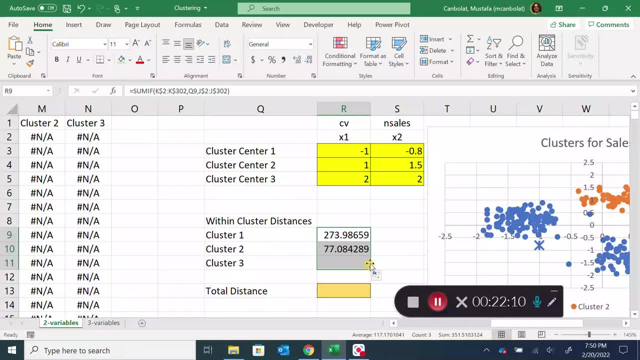 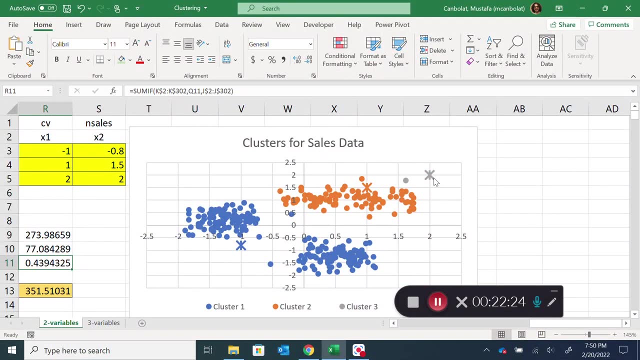 and 273 and 77 and 0.43. so why do you think that the cluster 3 has very small total distance within cluster distance, indicating that it only goes and grabs this point and that's the only distance. there is no other point as far as i can see there that's assigned to cluster three. so this total distance is 351. 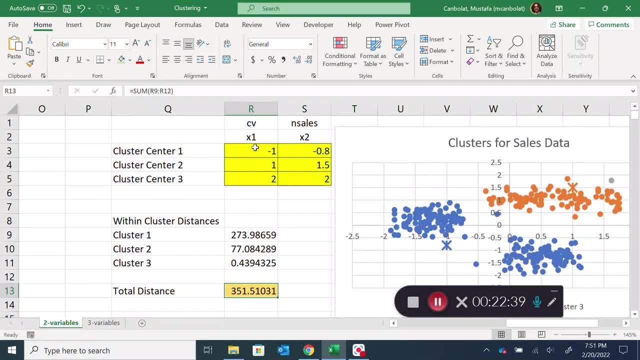 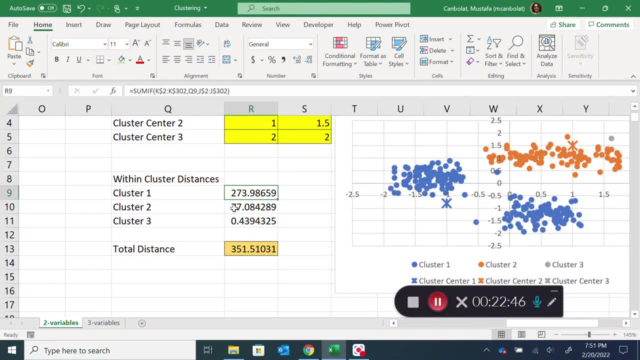 and this is not a correct distance. if i change this cluster center values and then the total distance is going to go down and every single one of this cluster distances will try to be lower, but the objective is just to lower the total of them and hold this. da gaughans, uh, you know algorithms. how did the algorithms do this? is that they are? 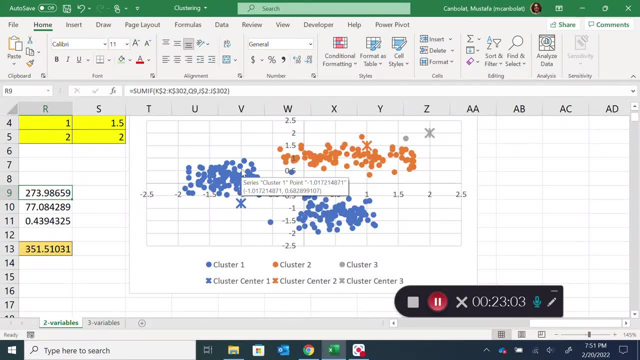 not using an optimization method that i'm going to be using here. they are using an iterative approach. so, for example, assume that these points are the initial point that they have selected as the center of these clusters and assigns these points to say that the center, and then what it does is find the center for this blue定. 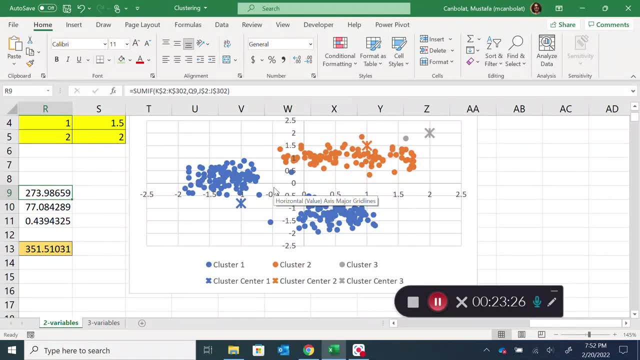 points which is not here. maybe it's going to be somewhere here and then find the center for the orange points. it's going to be somewhere here and then find a center point for the gray points. it's going to be some right on top of this gray point here. then it is going to look for the closest. 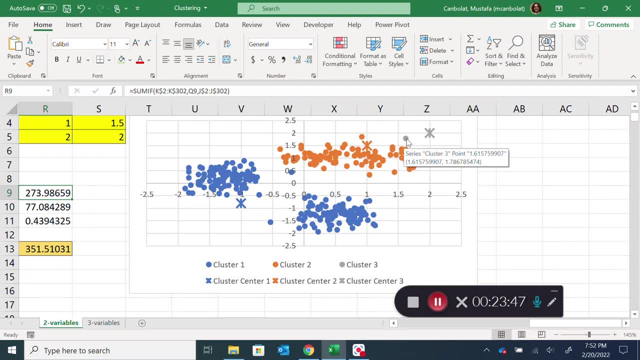 points to, to that new center, and it is going to be different from this, a new assignment. it is going to do that a multiple times in iterations and it is going to converge to the center and it is going to provide the best center for each cluster and it is going to minimize the 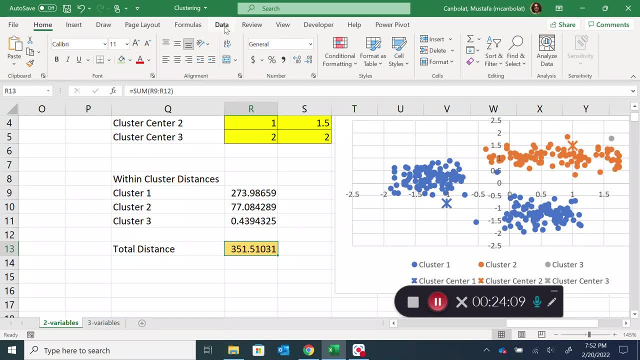 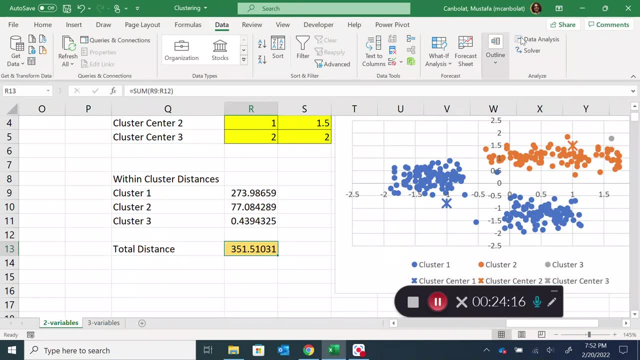 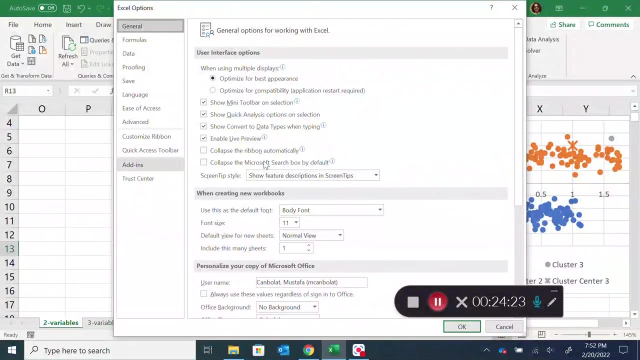 total distance. so how can we do? that is ourselves here. we are not going to write a macro to do that or something. we are going to use the solver and under the data tab there is solver. if it is not there, go to file more and options and then go to add-ins and under add-ins, excel add-ins, then go and just 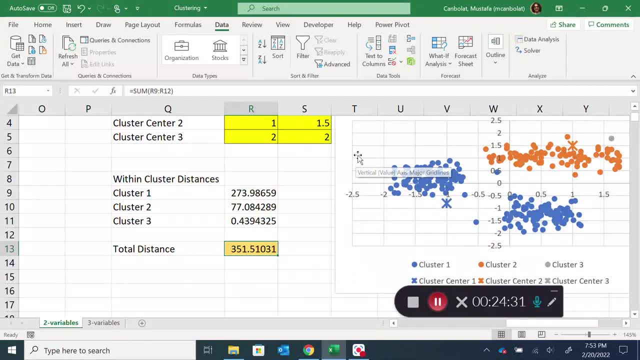 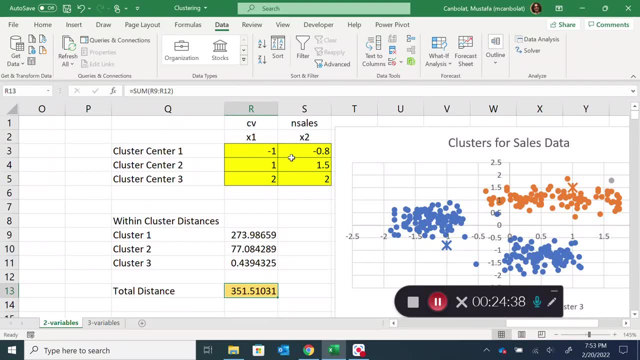 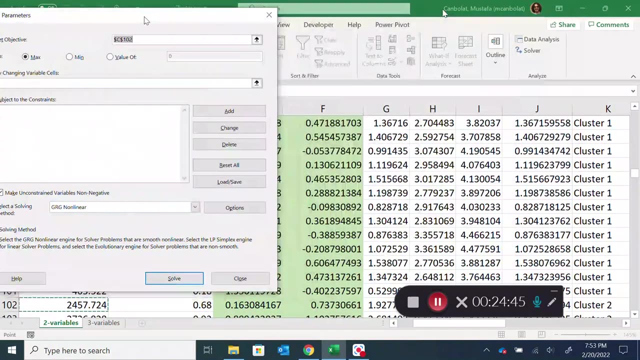 activate the solver add-in. if you have a mac computer, god bless. you just go to google and do a solver for mac computers and you will be able to find the solver how to install it. so once you have the solver in, we are going to have the solver menu there and in the solver. 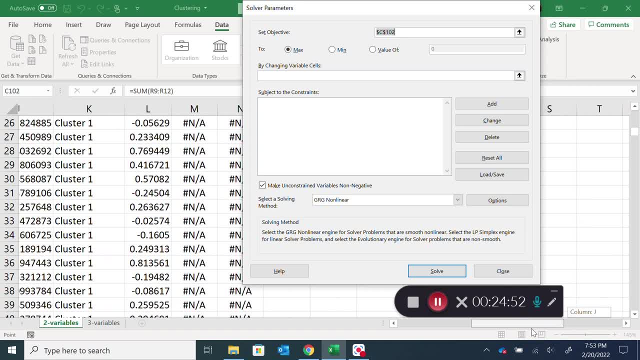 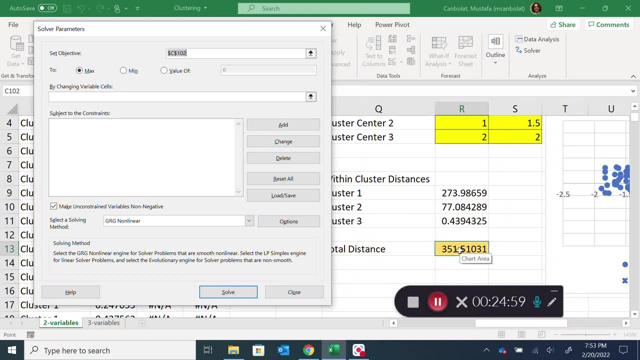 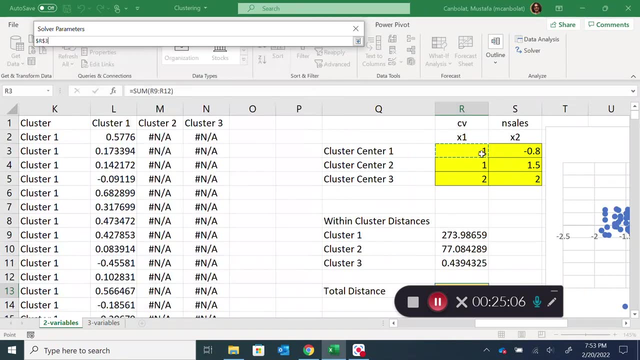 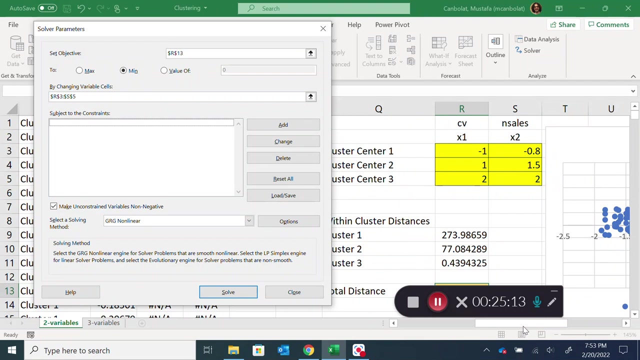 menu. what we're going to do is we are going to just use the- the total distance here, and just click on that r13. we want to minimize that by changing these six variables and then we are going to add a constraint to these variables. we know that the range of 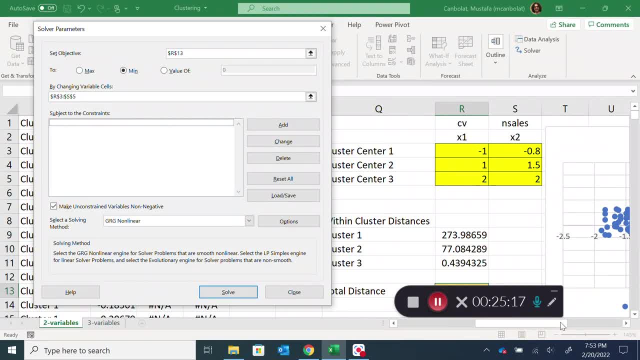 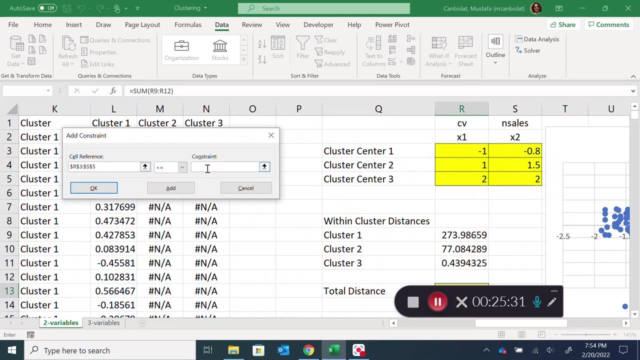 these variables right, so they are like going into negative two in there, and maybe let's just add some limits so that the solver will not look for extreme values. so we could. what we could say is that all of these are, we want them to be less than or equal to. let's say we could just directly say the maximum of the of. 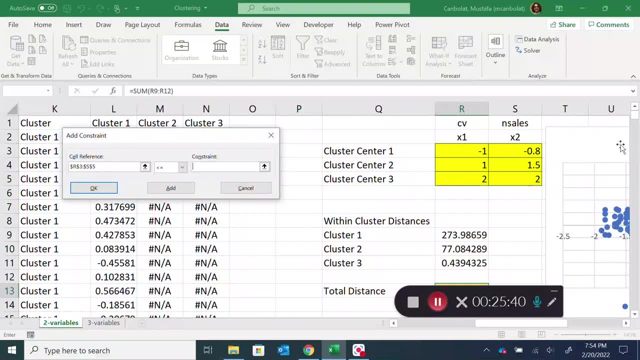 the values there that we are seeing in the coordinate axis, but I'm gonna just put five. okay, they have to be less than or equal to five. I could put four, and then I could put five, and then I could put five, and then I could put four too, because it's not going up to four, and then I'm gonna add that and I. 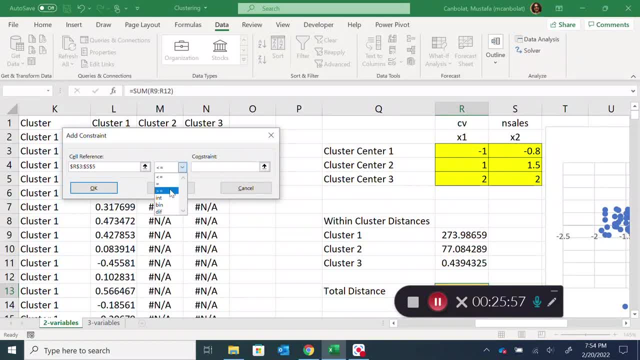 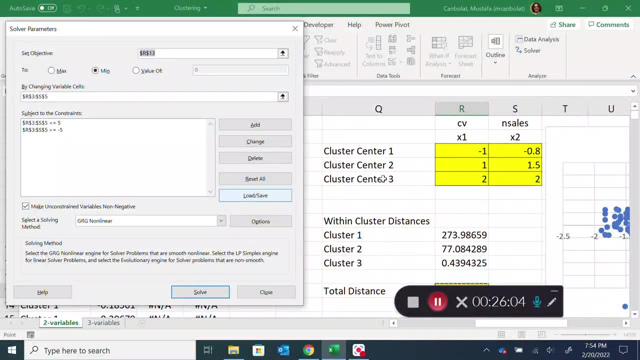 also want these points to be greater than or equal to negative five, then okay, and I do not want my variables to be non-negative, so I may be able to get the negative values there. and the final thing I want to do is I want to choose the evolutionary solver, because we have used some if statements there and some. 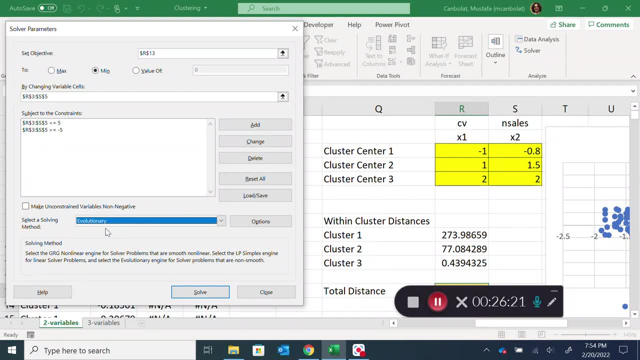 other things. I'm going to use the evolutionary solver because we have used some if statements there and some other things. I'm going to use the evolutionary solver because we have used some if statements there and some other things. a regular nonlinear solver is not going. things: a regular nonlinear solver is not going. 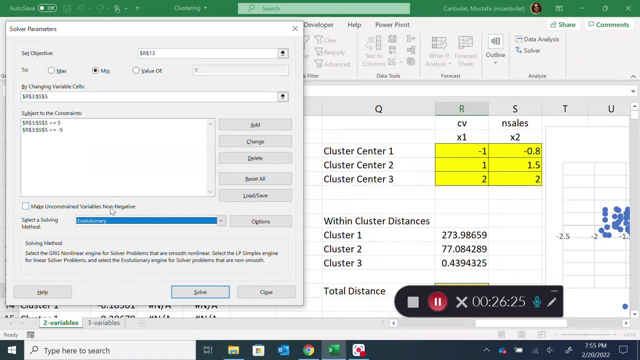 things. a regular, nonlinear solver is not going to be able to find us a solution, to be able to find us a solution, to be able to find us a solution, and even the evolutionary solver may not, and even the evolutionary solver may not, and even the evolutionary solver may not give us the best solution here. but 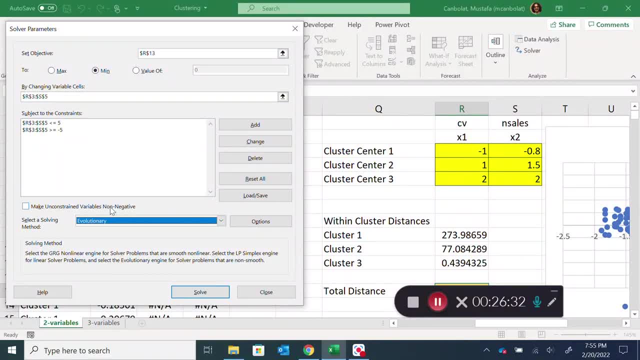 give us the best solution here. but give us the best solution here, but because it's a small problem, it is going because it's a small problem. it is going, because it's a small problem, it is going to provide us the best solution. it's to provide us the best solution. it's. 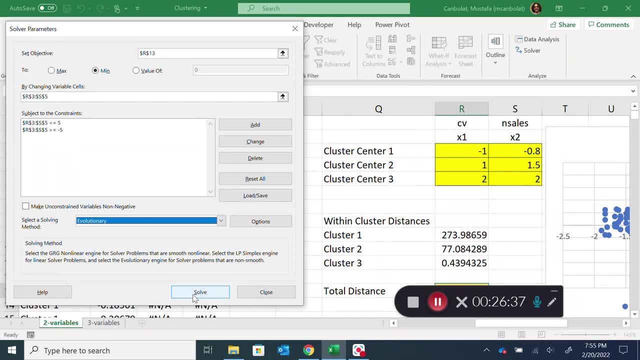 to provide us the best solution. it's already 26 minutes, oh my god, okay. so I'm already 26 minutes. oh my god, okay. so I'm already 26 minutes. oh my god, okay. so I'm gonna click on solve and hope for the. gonna click on solve and hope for the. 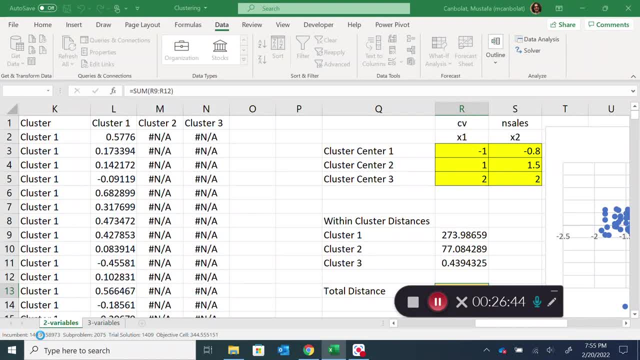 gonna click on solve and hope for the best as you see here, best as you see here, best as you see here. the the, the evolutionary solver is just going around. evolutionary solver is just going around. evolutionary solver is just going around and trying to find the best solution. it. 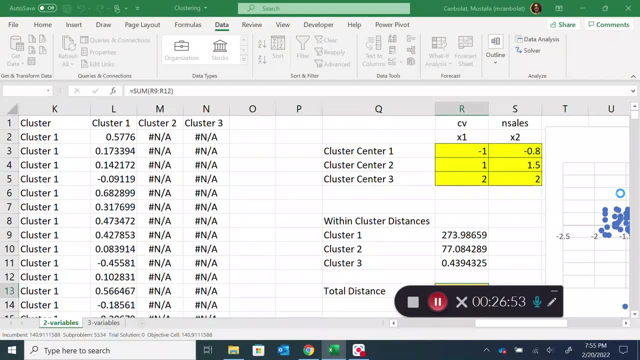 and trying to find the best solution. it and trying to find the best solution. it is trying to is trying to, is trying to minimize that total distance, minimize that total distance, minimize that total distance and it is going to converge after a and it is going to converge after a. 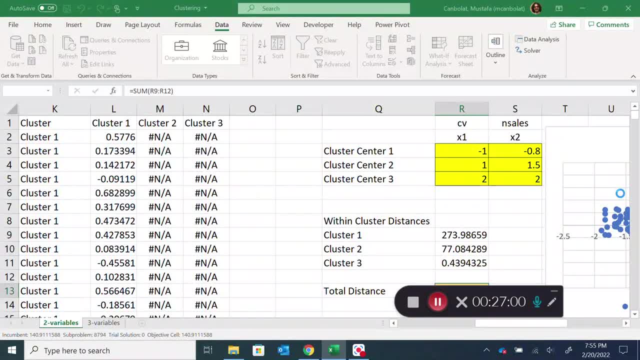 and it is going to converge after a while. it looks like it did converge, while it looks like it did converge, while it looks like it did converge to that 140.9 something value to that 140.9 something. value to that 140.9 something value, and it is still looking for mutating the 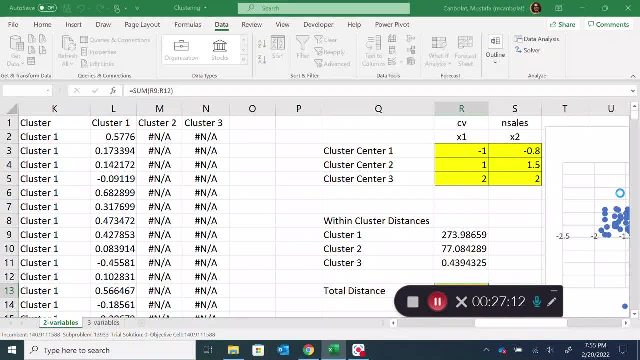 and it is still looking for mutating the and it is still looking for mutating the, the solution space, and it is trying to the solution space and it is trying to the solution space and it is trying to find, maybe, find, maybe, find, maybe, if it's stuck at the local optimum. 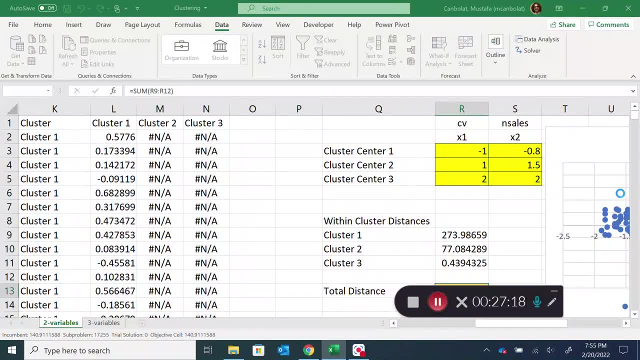 if it's stuck at the local optimum. if it's stuck at the local optimum, then it is going to try to escape from then. it is going to try to escape from then. it is going to try to escape from the local optimum by just trying the local optimum, by just trying. 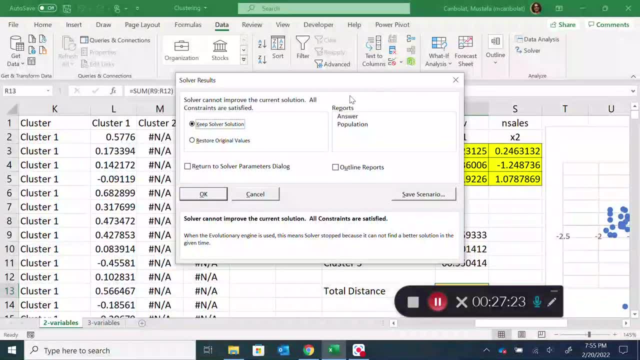 the local optimum by just trying, searching for other things, searching for other things, searching for other things. and it says it cannot improve the and it says it cannot improve the and it says it cannot improve the current solution. and we are able to find current solution, and we are able to find. 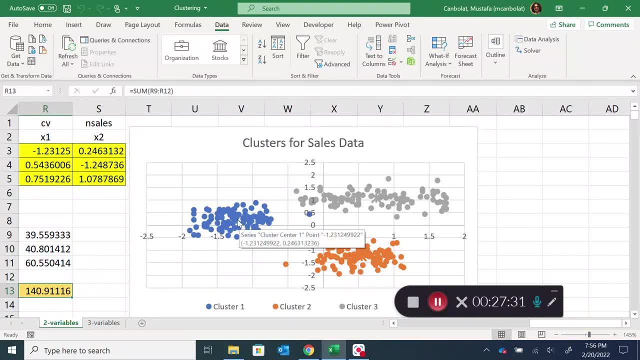 current solution and we are able to find the best solutions here. so we are able, the best solutions here, so we are able, the best solutions here, so we are able to find the best here, the center there, to find the best here, the center there, to find the best here, the center there and center there. they are hidden and 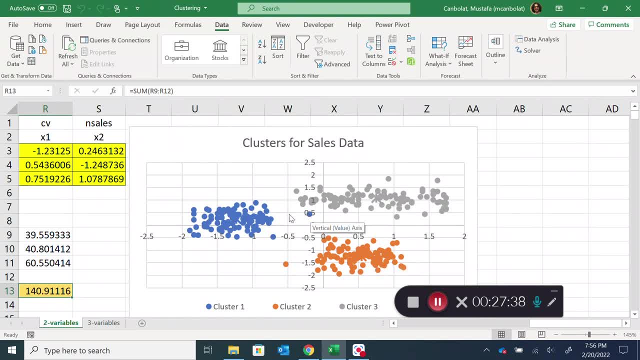 and center there they are hidden. and. and center there they are hidden. and center there, center there, center there. and it looks like this blue point is, and it looks like this blue point is, and it looks like this blue point is closer to this center than this center. 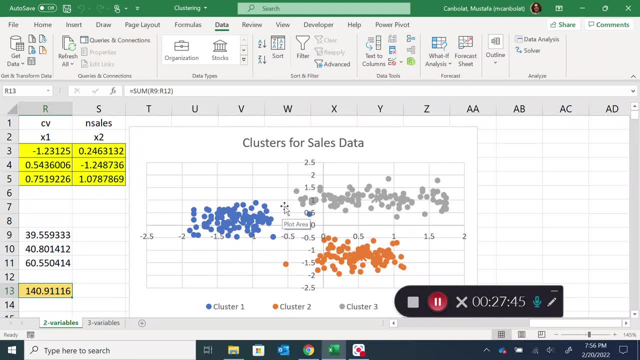 closer to this center than this center, closer to this center than this center. based on these values, based on these values. based on these values, so we were able to find the clusters for. so we were able to find the clusters for. so we were able to find the clusters for this. 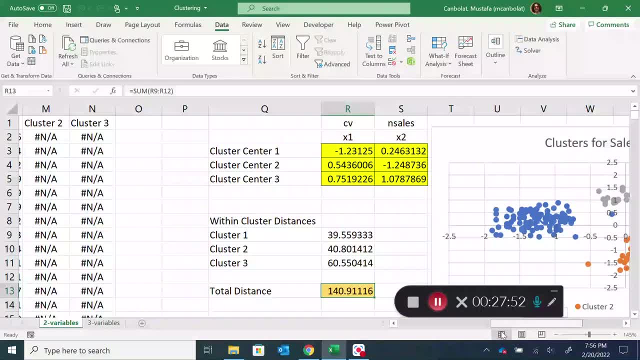 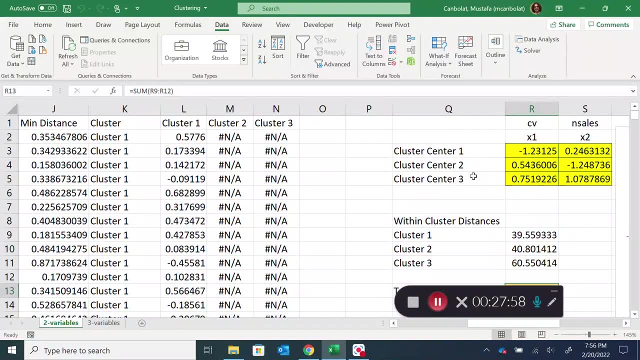 this, this, these observations, using three cluster these observations, using three cluster these observations, using three cluster centers for these observations, centers for these observations, centers for these observations, and these are the cluster centers and these are the cluster centers and these are the cluster centers for the for the. 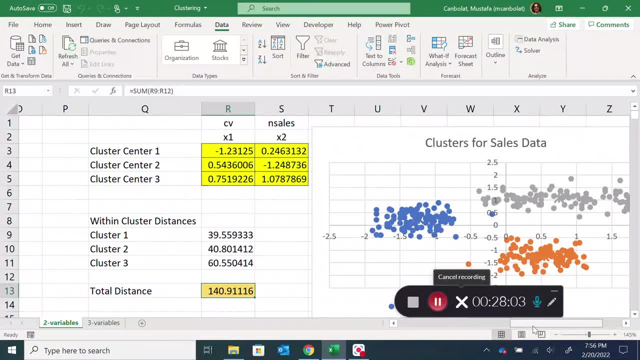 for the: modified for the normalized uh variables. modified for the normalized uh variables. modified for the normalized uh variables. okay, so the observation values there. okay, so the observation values there. okay, so the observation values there. now let's just look at this data. now, let's just look at this data. 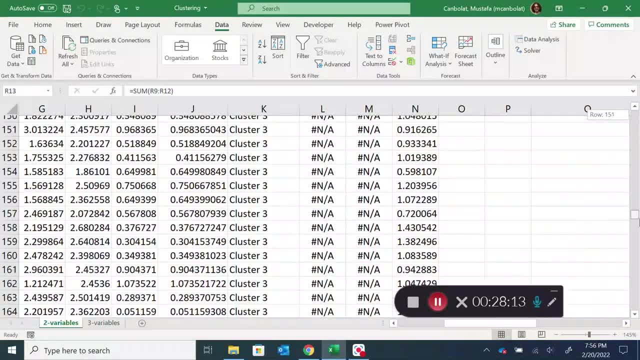 now let's just look at this data. this is the clusters that we want, right? this is the clusters that we want, right? this is the clusters that we want, right? we have the clusters one, two and three. we have the clusters one, two and three. we have the clusters one, two and three there. 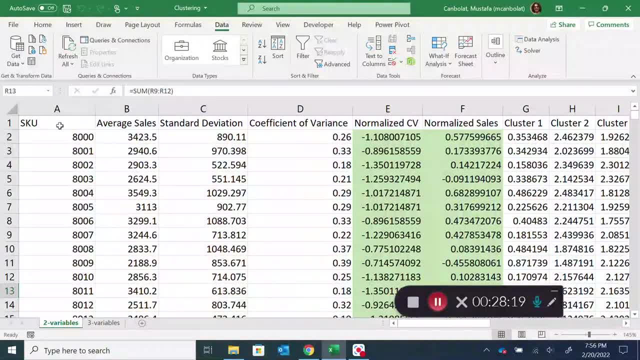 there, there, and what we want is we are going to now, and what we want is we are going to now, and what we want is we are going to now go to go to go to this stock keeping unit and we're going to this stock keeping unit and we're going to. 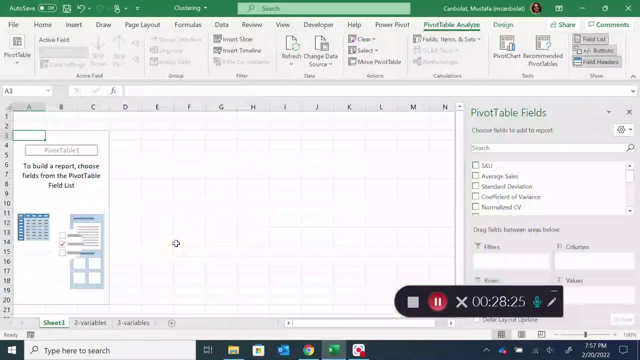 this stock keeping unit and we're going to insert a pivot table there. insert a pivot table there, insert a pivot table there, and and and we want to get in the pivot table. we want to get in the pivot table. we want to get in the pivot table. we want to put the cluster. 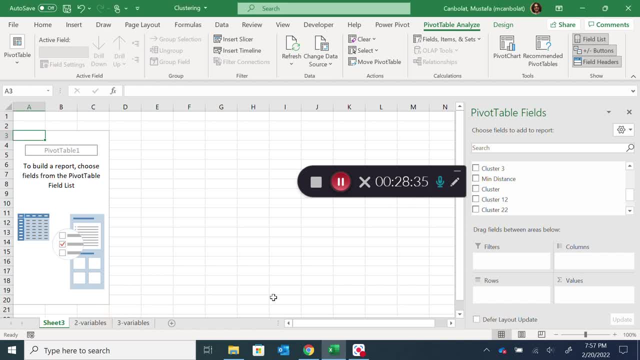 we want to put the cluster, we want to put the cluster. okay, where is that cluster thing for the okay, where is that cluster thing for the okay, where is that cluster thing for the two variables? two variables, two variables, and, and- and i want to just maybe get this only up to. 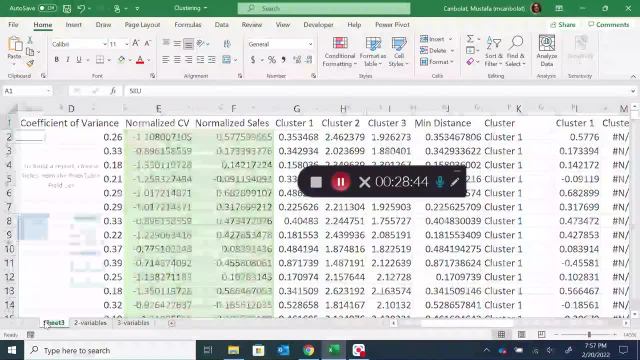 i want to just maybe get this only up to. i want to just maybe get this only up to the cluster. so i'm not going to just create this pivot table with every value, create this pivot table with every value, create this pivot table with every value there. 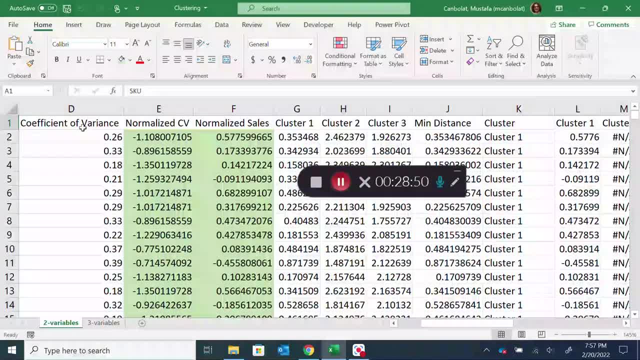 there, there. so let me just delete this pivot table. so let me just delete this pivot table. so let me just delete this pivot table here, here, here, and then i'm going to just highlight the, and then i'm going to just highlight the, and then i'm going to just highlight the stock keeping unit here. up to there. 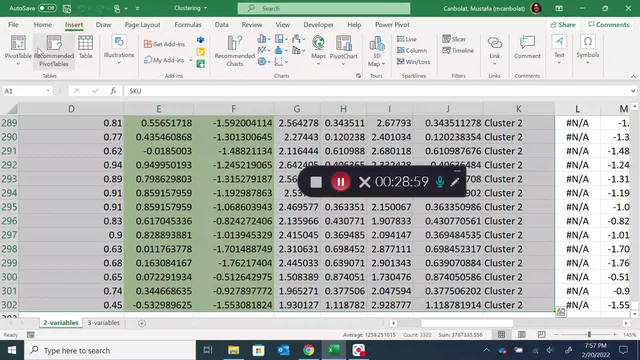 stock keeping unit here up to there, stock keeping unit here up to there, and then down and then down and then down. just select that data. just select that data. just select that data. insert a pivot table for that specific insert. a pivot table for that specific. insert a pivot table for that specific region in a new worksheet. 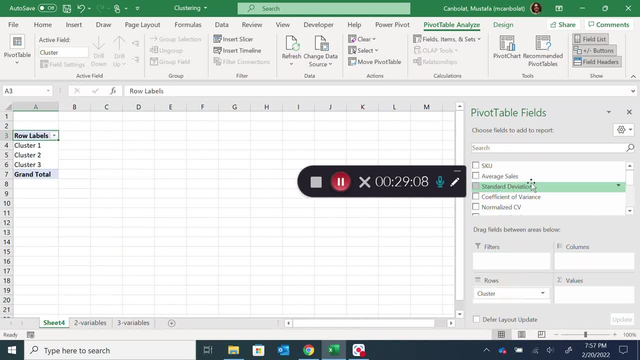 region in a new worksheet. region in a new worksheet and i take the cluster and i take the cluster and i take the cluster and i have three clusters there and i and i have three clusters there and i and i have three clusters there and i want to look at the average sales. 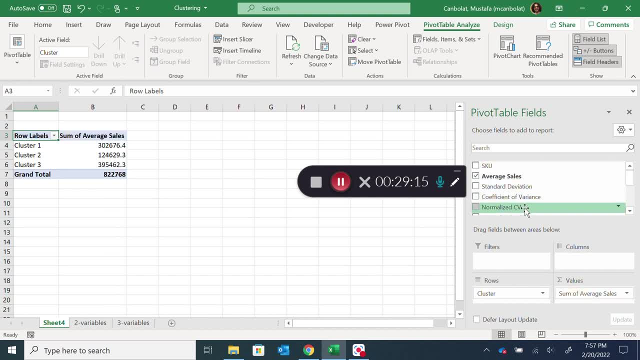 want to look at the average sales. want to look at the average sales? okay, okay, okay. and then i want to look at this standard, and then i want to look at this standard, and then i want to look at this standard: deviation or the coefficient of variance. deviation or the coefficient of variance. 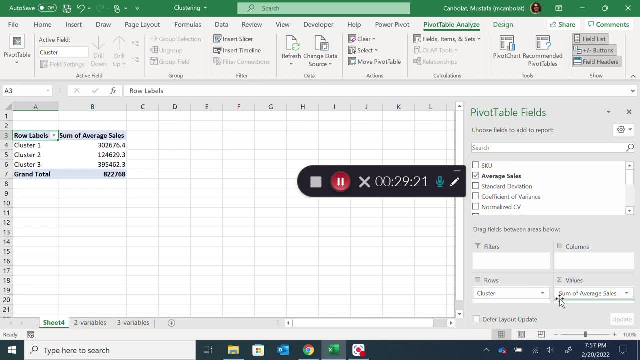 deviation or the coefficient of variance. let me just look at the coefficient of. let me just look at the coefficient of. let me just look at the coefficient of variance values and the standard variance values and the standard variance values and the standard deviation there. deviation there, deviation there. okay. 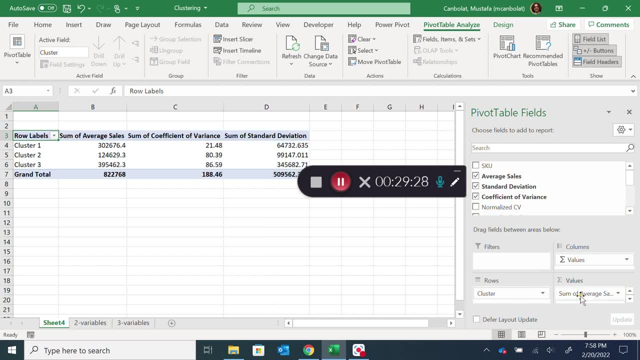 okay, okay, and and and. instead of finding the sum of those, instead of finding the sum of those, instead of finding the sum of those, i want to look at the- the averages. i want to look at the- the averages. i want to look at the- the averages. and the same thing for here, the averages. 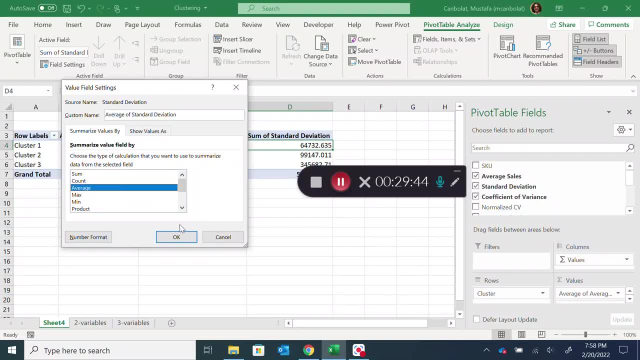 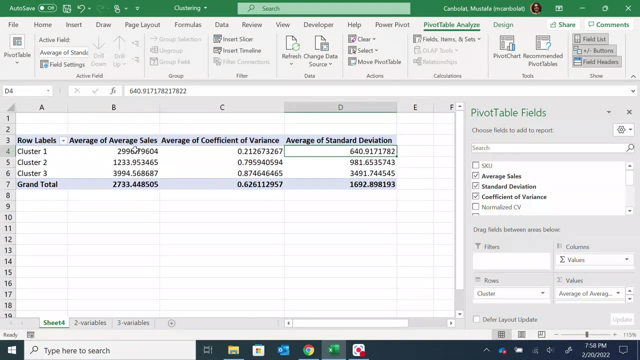 and the same thing for here, the averages, and the same thing for here, the averages, and then the same thing for here, the, and then the same thing for here, the, and then the same thing for here, the averages. so, so, so, let's, let's, let's focus on the, the average sales in each. 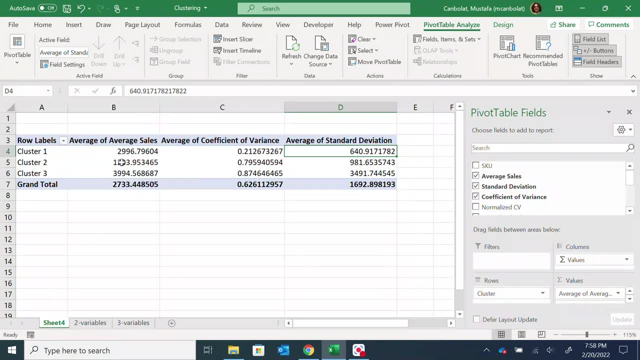 focus on the. the average sales in each. focus on the. the average sales in each cluster and cluster and cluster and the coefficient of variance for each. the coefficient of variance for each. the coefficient of variance for each cluster. assume that you did not, you were cluster. assume that you did not, you were. 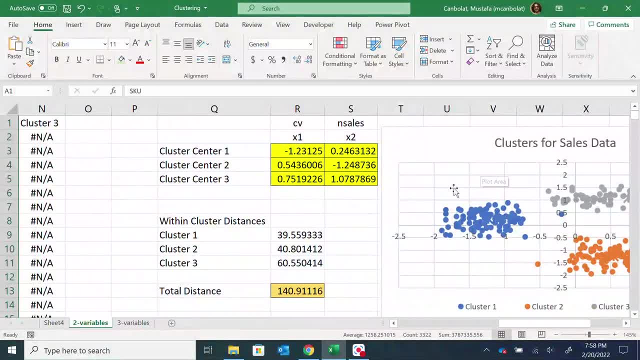 cluster. assume that you did not. you were not able to picture this in uh. not able to picture this in uh. not able to picture this in uh. let's say this is multiple, uh, multiple. let's say this is multiple, uh, multiple. let's say this is multiple, uh, multiple. variable space. 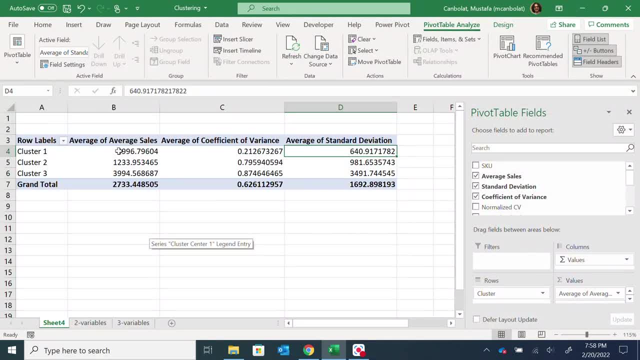 and you are not able to, and you are not able to and you are not able to visualize it. you can still look at these, visualize it. you can still look at these, visualize it. you can still look at these numbers and come up with certain numbers and come up with certain. 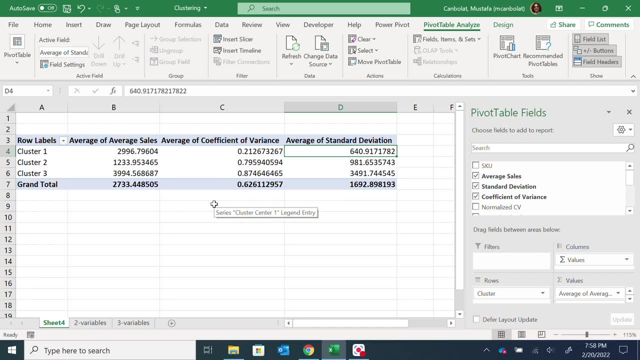 numbers and come up with certain conclusions, and you can develop certain conclusions, and you can develop certain conclusions and you can develop certain uh, maybe policies based on all these uh, maybe policies, based on all these uh, maybe policies, based on all these results, results, results. so what i see here is that 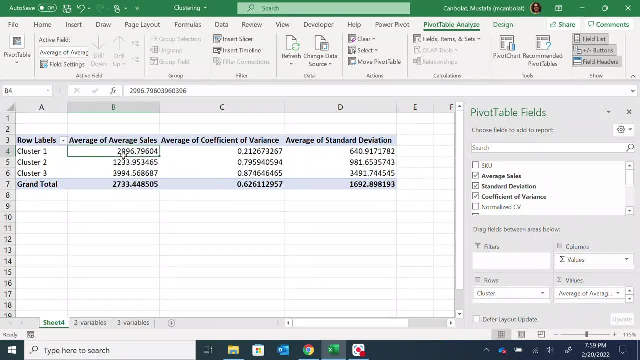 so what i see here is that. so what i see here is that i see that cluster one has kind of an. i see that cluster one has kind of an. i see that cluster one has kind of an average or on the higher and the sales average, or on the higher and the sales. 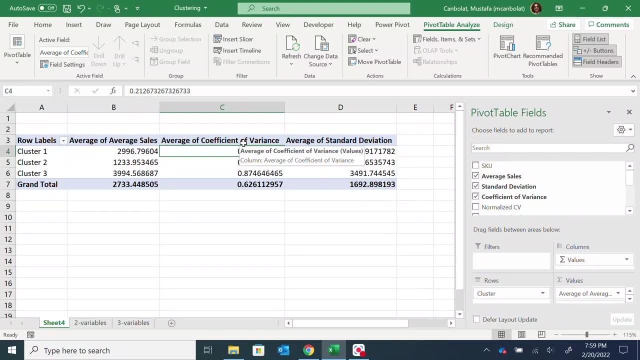 average or on the higher and the sales it has lower, it has lower, it has lower variance, variance variance for the sales. so this products for the sales, so this products for the sales, so this products. you have good sales amounts and then you. you have good sales amounts and then you. 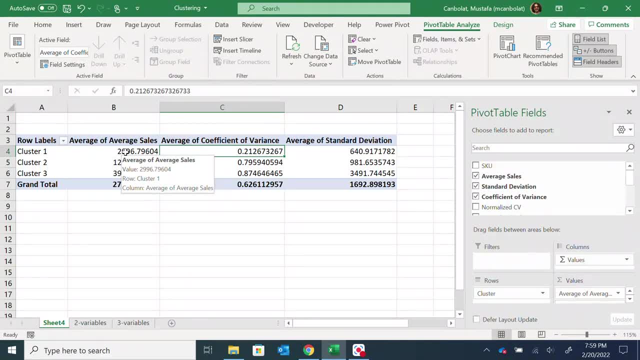 you have good sales amounts and then you have low variance in your sales amounts. have low variance in your sales amounts, have low variance in your sales amounts. those, these products are very valuable to those. these products are very valuable to those. these products are very valuable to you, right? so? 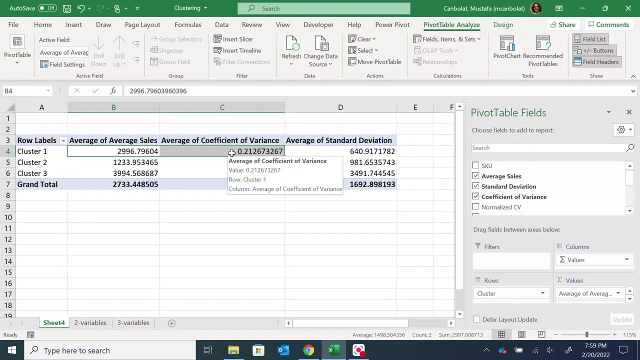 you right, so you right, so you know, you know. you know if you're going to be selling around. if you're going to be selling around, if you're going to be selling around 3 000 and these are the products that. if you're going to be selling around 3 000 and these are the products that. 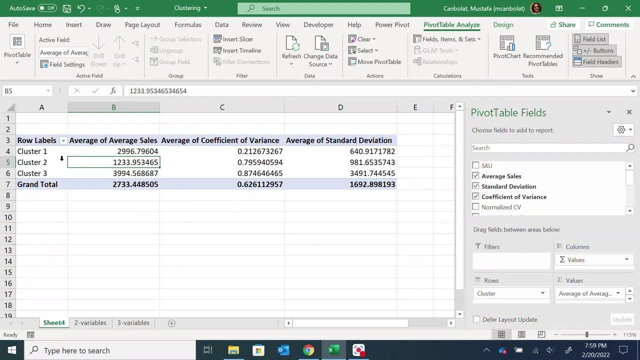 if you're going to be selling around 3 000, and these are the products that you want to pay attention to. you want to pay attention to, you want to pay attention to the second cluster, the, the second cluster, the, the second cluster, the. the sales are low and there there is a. 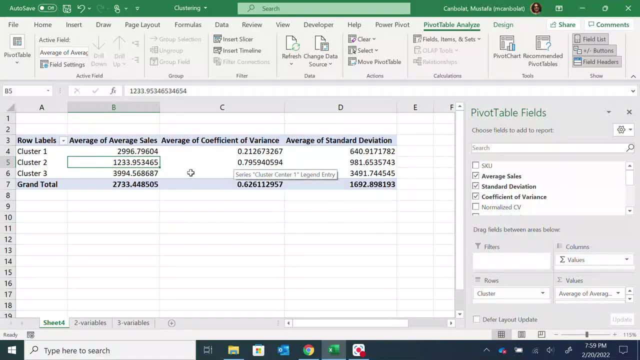 the sales are low and there there is a. the sales are low and there there is a large, large, large variance there, variance there, variance there. so these products are, so these products are, so these products are. you're not getting a lot of money from. you're not getting a lot of money from. 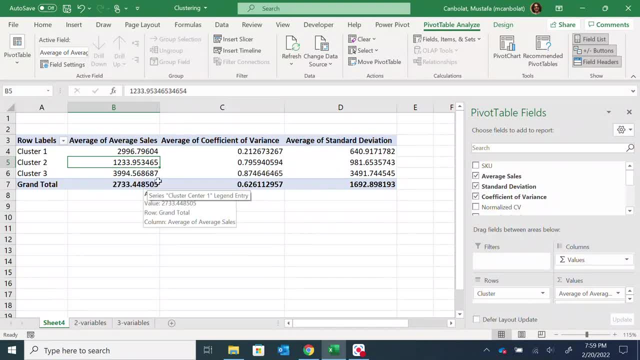 you're not getting a lot of money from these products, these products, these products, the average sales amounts, the average sales amounts, the average sales amounts, and, and and there's also, there's also. there's also a lot of variance. so sometimes you are a lot of variance, so sometimes you are. 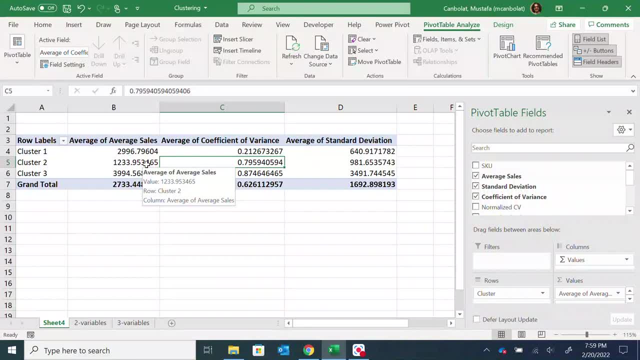 a lot of variance. so sometimes you are selling, selling, selling twelve hundred dollars on average, but twelve hundred dollars on average, but twelve hundred dollars on average. but sometimes you are selling much less and sometimes you are selling much less, and sometimes you are selling much less and much more. there's a 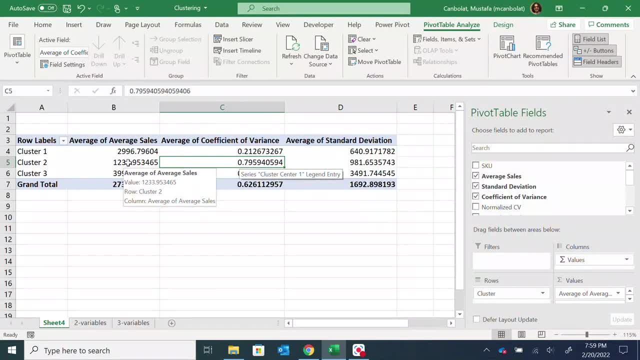 much more. there's a much more. there's a huge uh variance in there, but the huge uh variance in there, but the huge uh variance in there. but the average is on the lower side, average is on the lower side, average is on the lower side. and this cluster here, although you are, 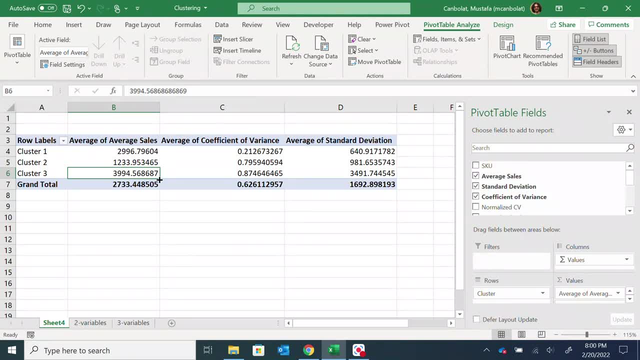 and this cluster here, although you are, and this cluster here, although you are having a lot of sales in here, having a lot of sales in here, having a lot of sales in here in terms of the dollar value, in terms of the dollar value, in terms of the dollar value, but you are also having, seeing uh. 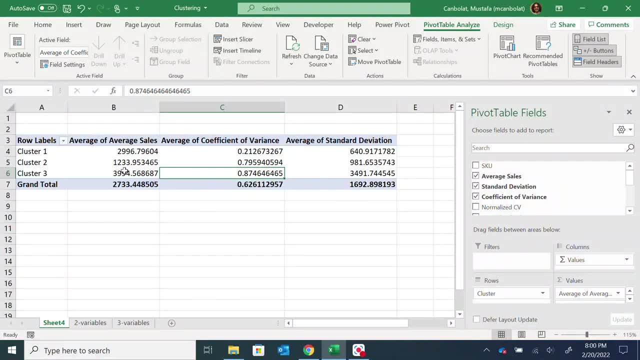 but you are also having seeing uh, but you are also having seeing uh, a large variance. so you are not really a large variance. so you are not really a large variance, so you are not really able to predict maybe able to predict, maybe able to predict, maybe the values for the product stock. 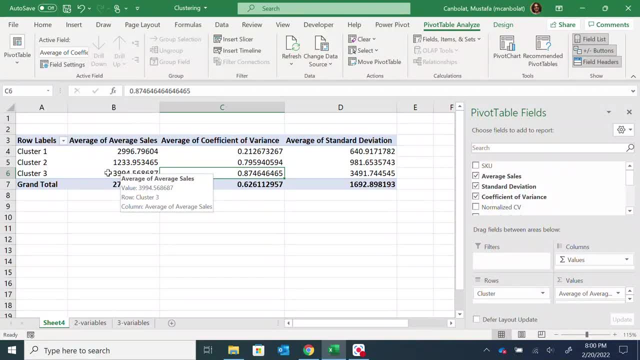 the values for the product stock. the values for the product stock: keeping units in the third cluster. keeping units in the third cluster, keeping units in the third cluster. because, because, because the numbers are, the numbers are. the numbers are just in, uh, just in, uh, just in uh, close to like 87 percent of them. 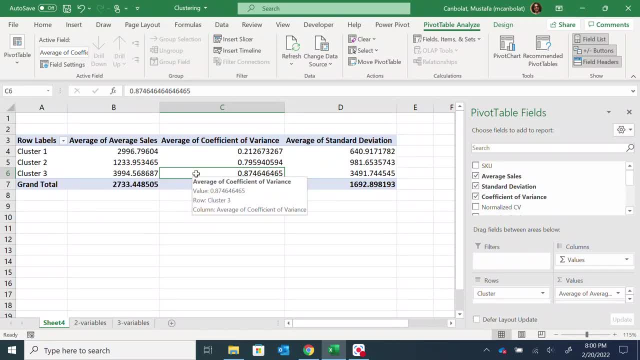 close to like 87 percent of them. close to like 87 percent of them. uh of the sales amount is the coefficient uh of the sales amount is the coefficient uh of the sales amount is the coefficient of variance right. so of variance right, so of variance right. so standard deviation is very high. 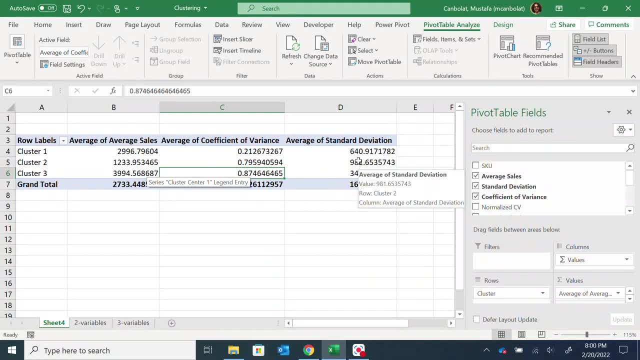 standard deviation is very high. standard deviation is very high and uh and uh and uh, as you see here, 981 is kind of not really as you see here, 981 is kind of not really. as you see here, 981 is kind of not really telling you the truth, because 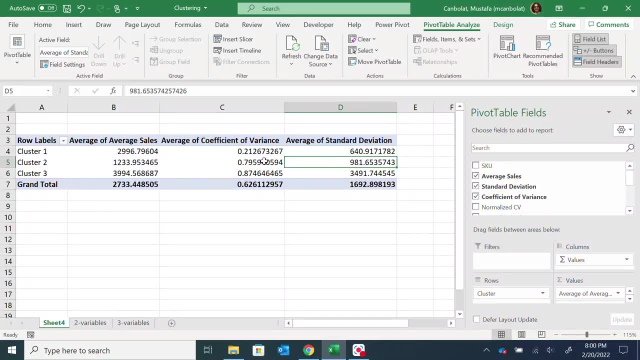 telling you the truth, because telling you the truth, because this is depend based on the. this is depend based on the. this is depend based on the. the average here is 0.79. the average here is 0.79. the average here is 0.79. this is a better number to look at, rather. 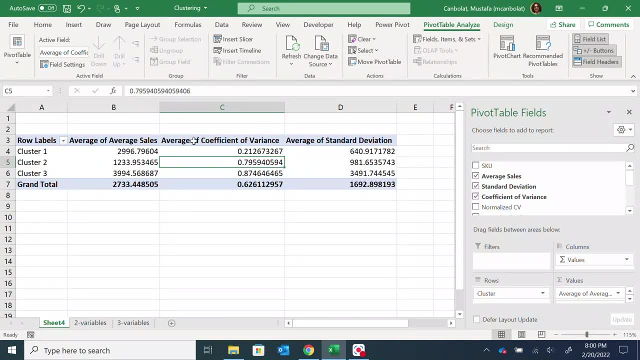 this is a better number to look at. rather, this is a better number to look at rather than looking at the standard deviation, than looking at the standard deviation, than looking at the standard deviation itself itself itself. so now we are seeing that there are. so now we are seeing that there are. 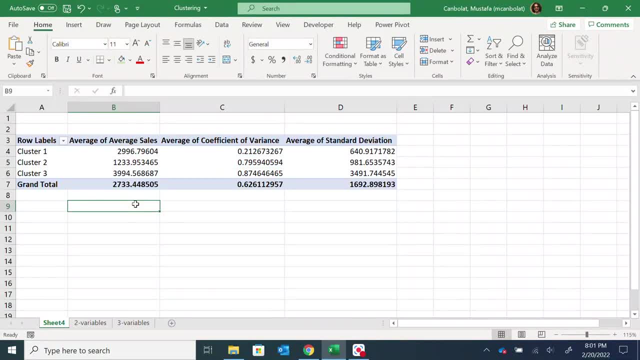 so now we are seeing that there are three distinct groups and we can maybe three distinct groups and we can maybe three distinct groups and we can maybe treat these different types of products, treat these different types of products, treat these different types of products in a different way. 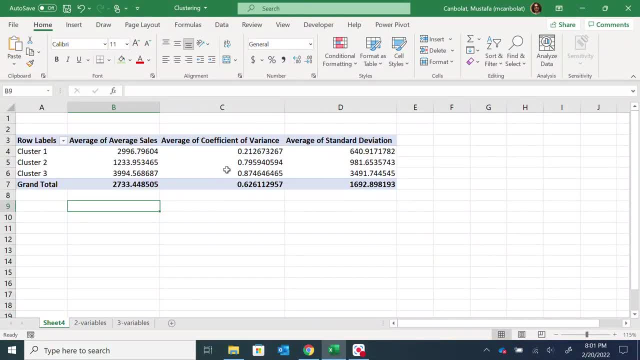 in a different way, in a different way, and i can maybe look at cluster three and i can maybe look at cluster three, and i can maybe look at cluster three and and, and just just just look at this cluster group, look at this cluster group, look at this cluster group and let me just look at which products are. 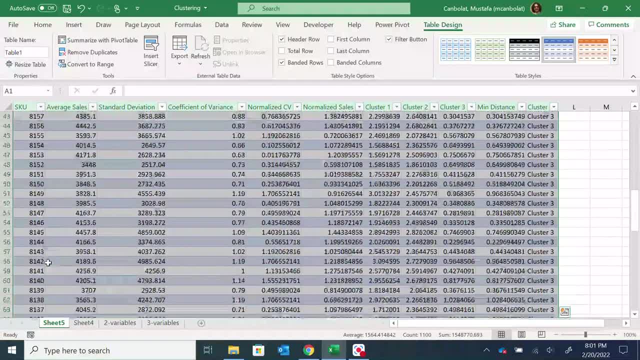 and let me just look at which products are and let me just look at which products are they. they are these products, they, they are these products, they, they are these products and i can focus more on these products and i can focus more on these products and i can focus more on these products here. 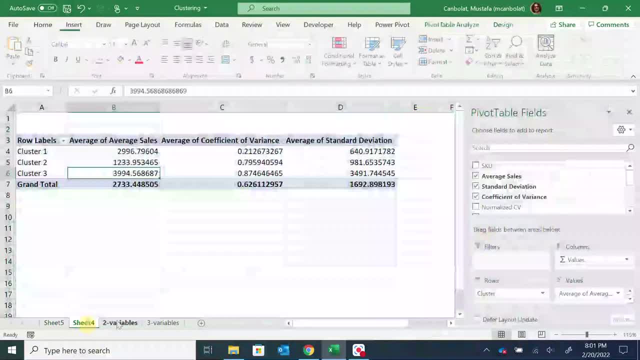 here, here, and because they are having having higher, and because they are having having higher and because they are having having higher sales, sales, sales, and i know that i don't need to worry a and i know that i don't need to worry a and i know that i don't need to worry a lot about cluster one. 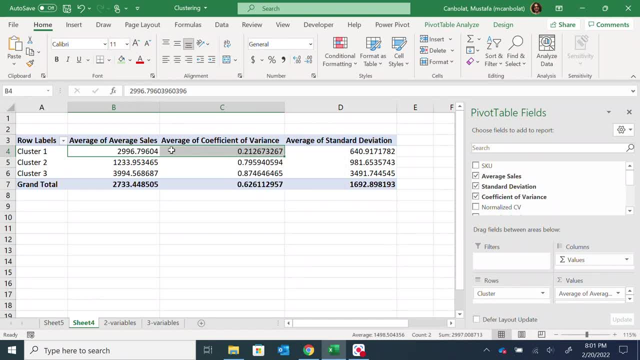 lot about cluster one. lot about cluster one because i, because i, because i am going to be able to estimate or predict, am going to be able to estimate or predict, am going to be able to estimate or predict the sales for this cluster, the sales for this cluster. 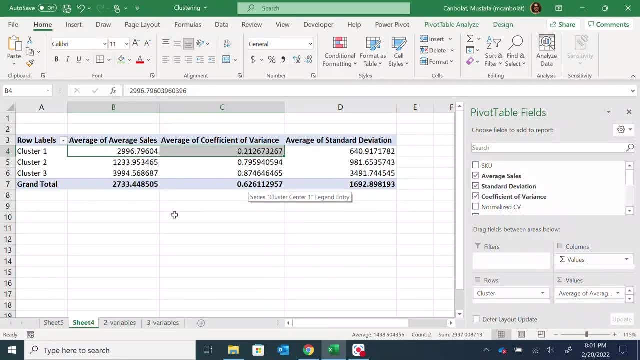 the sales for this cluster better than the others. because there's a better than the others, because there's a better than the others because there's a lower variance in there, lower variance in there, lower variance in there. okay, so this is done for what this is. okay, so this is done for what this is. 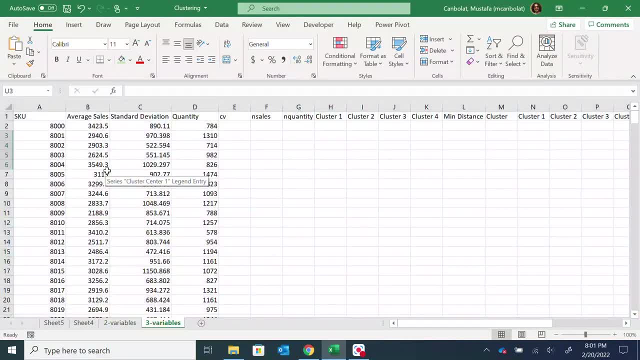 okay, so this is done for what? this is done for two variables and we can also do done for two variables and we can also do done for two variables and we can also do that for three variables. i'm going to that for three variables, i'm going to. 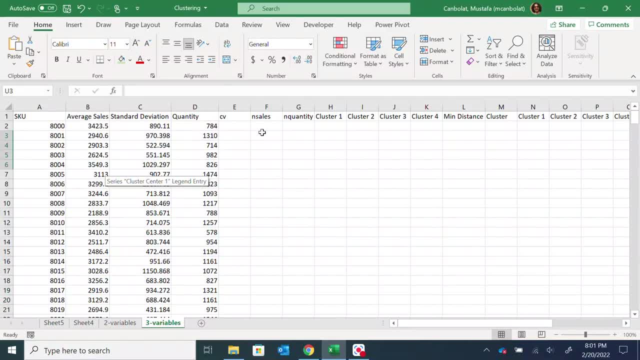 that for three variables. i'm going to just keep it in here. i'm not going to just keep it in here. i'm not going to just keep it in here. i'm not going to solve this, but i recommend you to solve this, but i recommend you to. 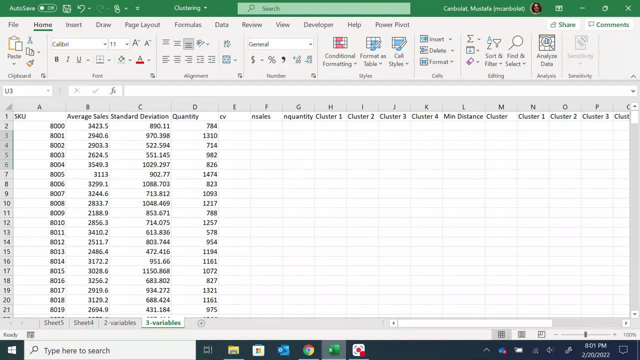 solve this, but i recommend you to work on this and find the work on this, and find the work on this and find the. find the total. find the total. find the total uh distance for four clusters. uh distance for four clusters. uh distance for four clusters using three variables. so the sales. 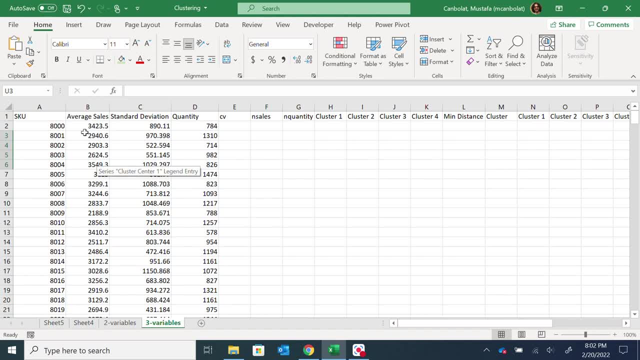 using three variables. so the sales using three variables. so the sales: standard deviation and quantity now. so standard deviation and quantity now. so standard deviation and quantity now. so this is the sales amount, this is the sales amount. this is the sales amount in terms of the dollar value and the 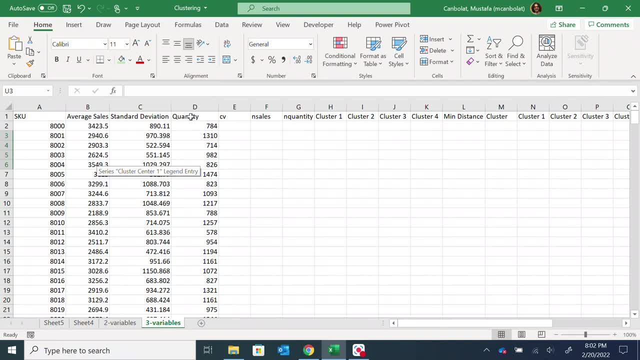 in terms of the dollar value and the in terms of the dollar value and the standard deviation of that dollar value, standard deviation of that dollar value, standard deviation of that dollar value. and these are the number of sales in and these are the number of sales in and these are the number of sales in here. 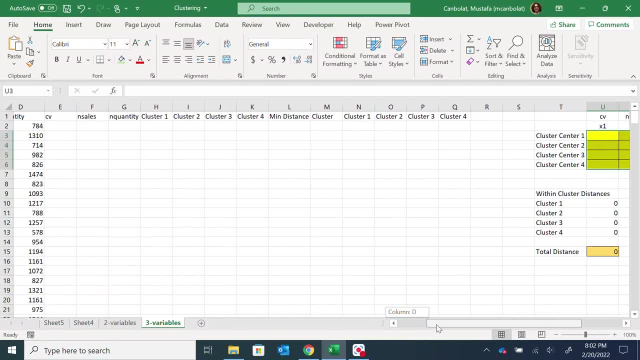 here, here, and using this three, and using this three, and using this three, uh columns, uh columns, uh columns. would you be able to come up with the? would you be able to come up with the? would you be able to come up with the minimum total distance, once you find that? 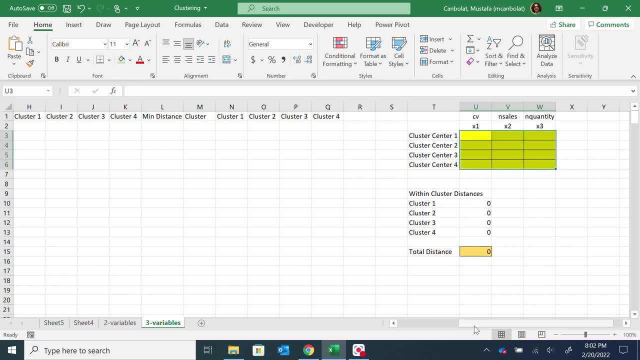 minimum total distance. once you find that minimum total distance, once you find that, you can put that in your comments and you can put that in your comments, and you can put that in your comments and let's see if everyone is going to get. let's see if everyone is going to get. 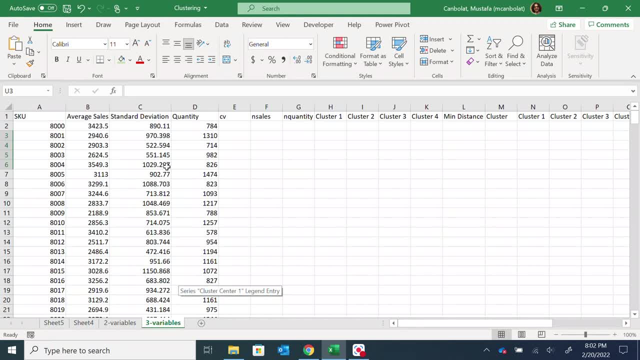 let's see if everyone is going to get the same values, the same values, the same values. in the next video i'm going to show you. in the next video i'm going to show you. in the next video, i'm going to show you how to do. 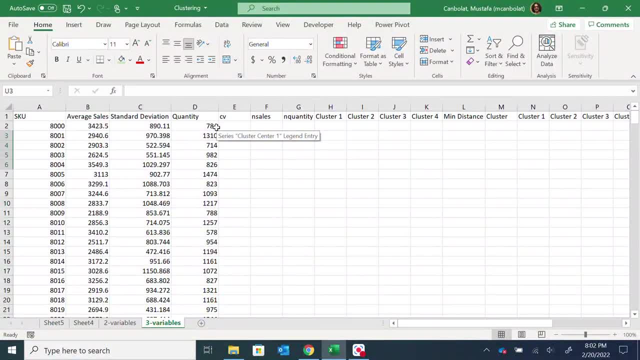 how to do, how to do two variable and three variable, two variable and three variable, two variable and three variable, clustering, clustering, clustering using power bi and then r using power bi and then r using power bi and then r. you can compare, uh, the efficiency of. you can compare, uh, the efficiency of. 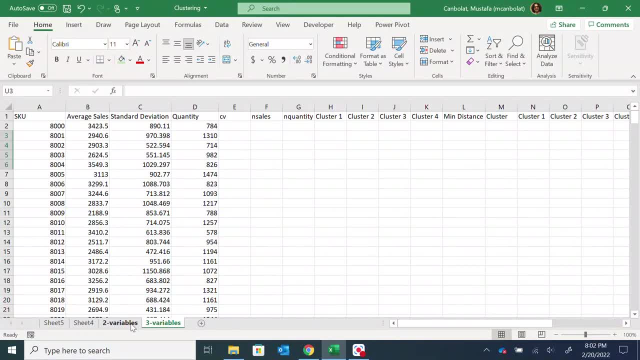 you can compare, uh, the efficiency of the the methods and the r is the most, the the methods and the r is the most the the methods and the r is the most efficient, efficient, efficient one, and the power bi is more i think the one and the power bi is more i think the.